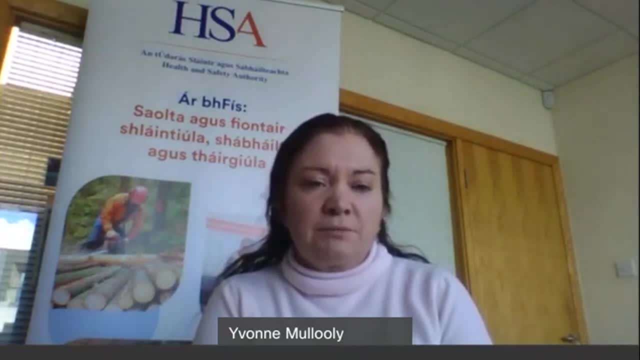 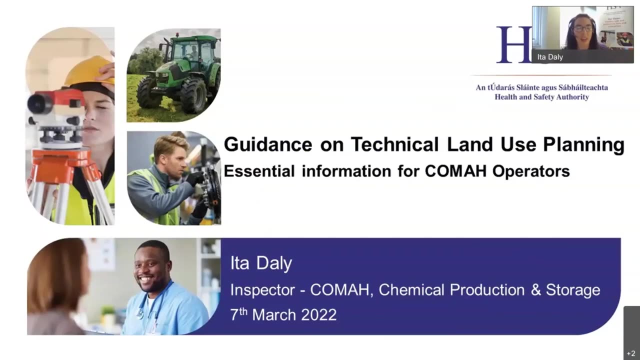 So I'll pass you over now to Eita. So thank you to Yvonne for the introductions and good morning everyone. I too would like to welcome you all to this webinar on our recently launched guidance on technical land use planning And, as Yvonne mentioned, this webinar is being recorded so it will be available on the authority's website in due course for any of your colleagues who are unable to join us this morning. We will have time to answer your questions at the end of the presentations, and these can be submitted using the Q&A function. 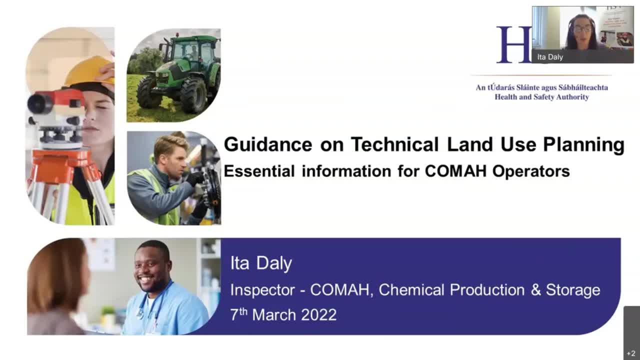 If you have any questions at the end of the presentations, and these can be submitted using the Q&A function. If you have any questions at the end of the presentations, and these can be submitted using the Q&A function at the bottom right of your screen. 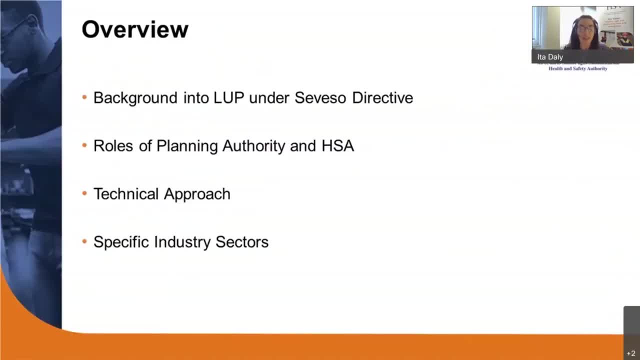 Just by way of introduction, my name is Eta Daly and I'm an inspector in the coma unit based here in the Cork office. As well as carrying out inspections and other coma regulatory duties, such as safety report and notification assessment, my colleagues and I are also tasked. 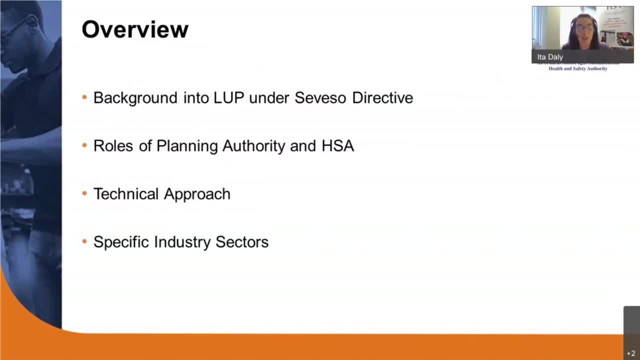 with providing technical advice in response to requests submitted to us by planning bodies for proposed development on or in the vicinity of a coma site. I'm going to cover that in a little bit more detail and how that relate backs to you as a coma site operator. 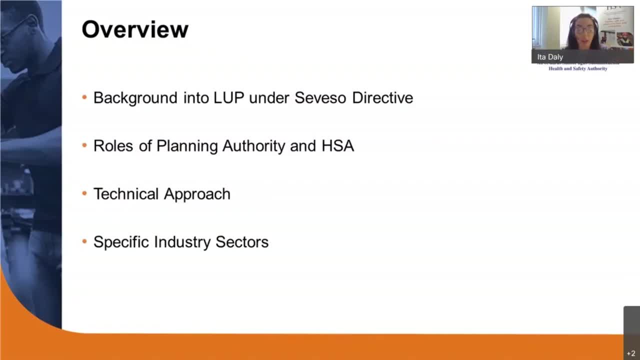 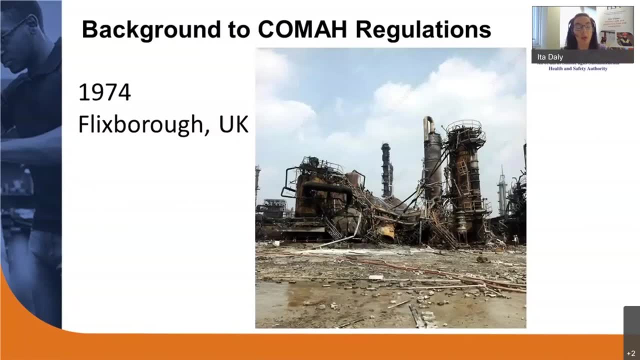 But first let's look at the requirement for how land use planning came about. So in the 1970s, the chemical industry was experiencing a period of exponential growth and the primary focus of most companies was to develop advanced chemical processes to fulfill the demand for new materials. 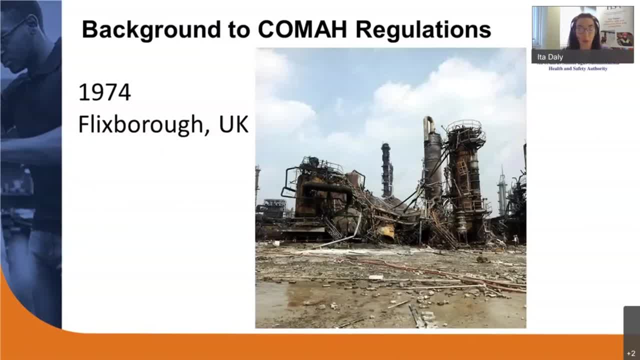 following the scientific technical revolution that began in the 1970s And after the Second World War. So there were a number of catastrophic industrial accidents as a result of this record growth in the chemicals industry, And one of those was an explosion at a chemical plant. 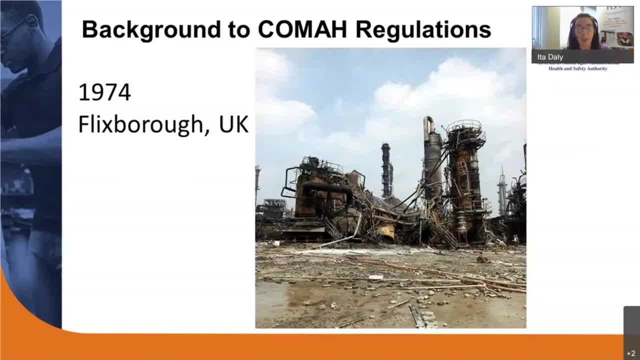 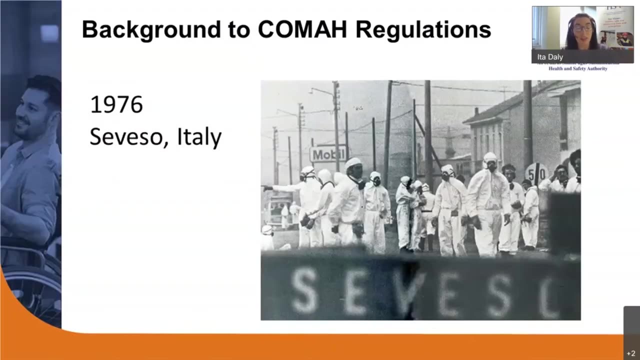 in Flixborough in the UK, killing 28 people and injuring 36 on the site. There were, additionally, there were 55 offsite injuries and up to 2000 homes and businesses in the vicinity suffered significant structural damage. In 1976, at a chemical plant near a town called Savais. 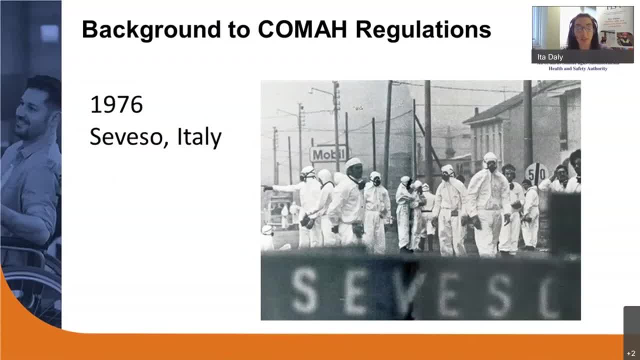 in Italy, a dense vapor cloud containing dioxin, which is both poisonous and carcinogenic, was released, resulting in more than 2000 people being treated for dioxin poisoning and the contamination of 10 square miles of land and vegetation. 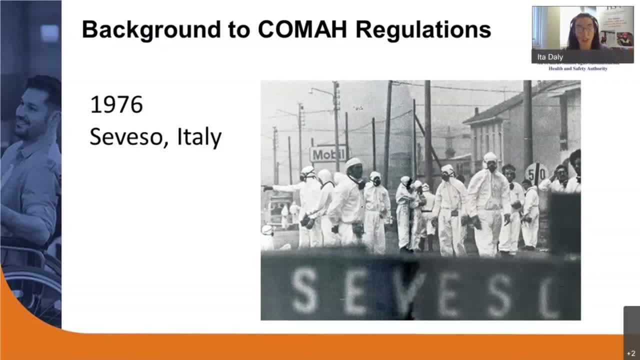 Events such as both of these incidents prompted the adoption of legislation on the prevention and control of such accidents in Europe, And hence came the so-called Savais 1 directive. The Savais 1 directive was then amended in view of the lessons learned from later accidents. 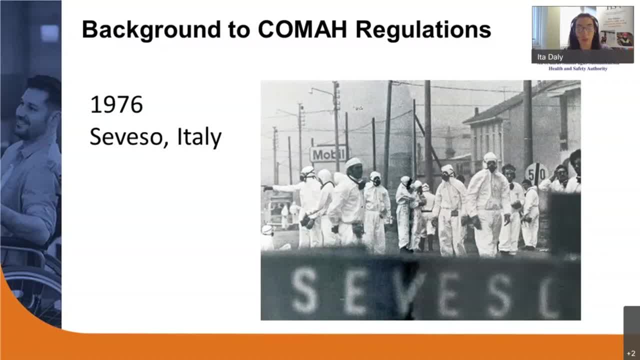 such as in Bhopal and Mexico City, and this brought about the Savais 2 directive, which introduced new requirements for land use planning. Most recently, the Savais 3 directive was adopted, and this took account of lessons learned from accidents. 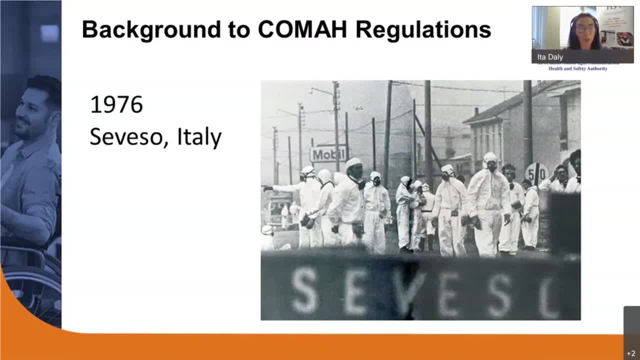 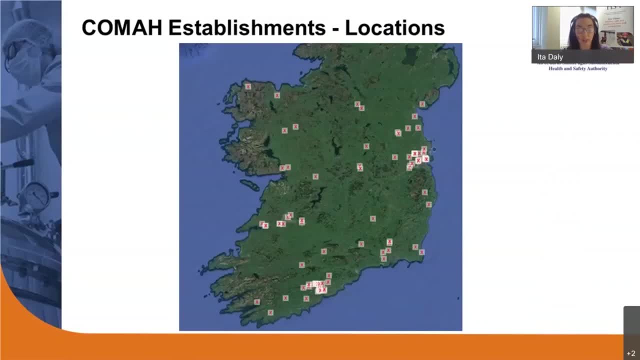 such as in Toulouse and Buncefield. So in Ireland the COMA or the Savais 3 directive is implemented by the Chemicals Act Control of Major Accident Hazards Involving Dangerous Substances Regulations, or COMA regulations in 2015.. 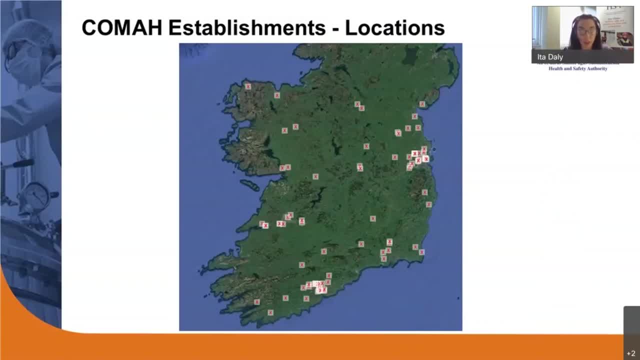 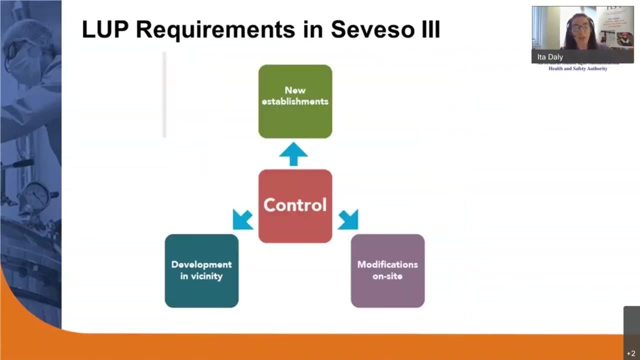 And it applies to about 100 establishments which, apart from a concentration in Cork and Dublin, are generally spread throughout the country, as you can see from the map here. So what are the land use planning requirements that apply to all these sites? So, the protection of residential and other populated areas. 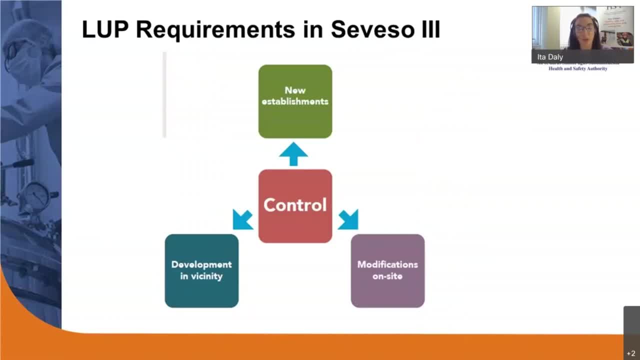 likely to be affected by a major accident is a key aim of the Savais 1 directive. It also covers the safeguarding of environmental receptors. So the directive sets out that member states should ensure that the objectives of preventing major accidents and limiting consequences of such accidents 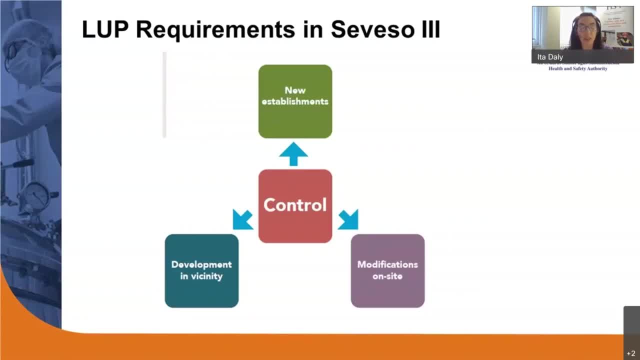 are taken account into their land use policies, And these objectives should be pursued through controls on three separate types of development. So firstly, the siting and development of new establishments, then modifications to existing establishments and finally, development in the vicinity of establishments. 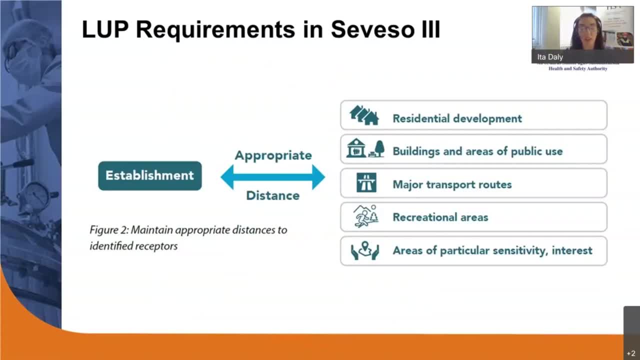 And in applying these controls, a count must be taken of the long-term requirement to maintain appropriate distances between establishments. And you can see the list here: residential areas, buildings and areas of public use, major transport routes and recreation areas and areas of particular natural sensitivity or interest. 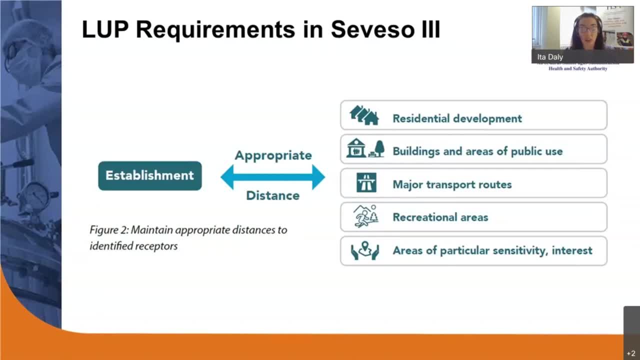 So, as I mentioned and as set out in the new guidance document, the Savais 1 directive is primarily implemented under the COMA regulations of 2015, and the land use planning requirements of the directive are addressed by Regulation 24.. In addition to the COMA regulations, 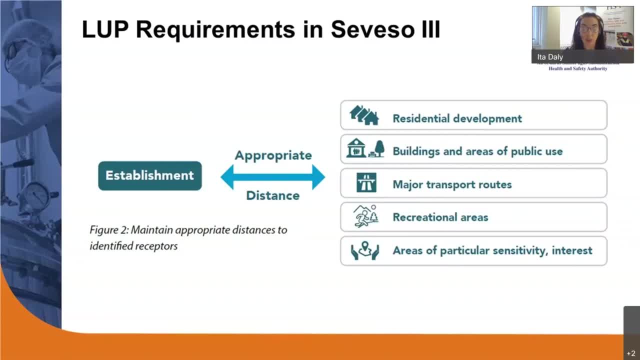 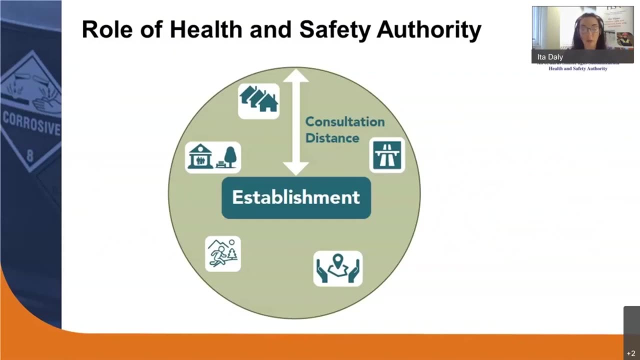 the planning and development regulations also play a part in the implementation of the directive, So let's now look at the roles of both the HSA and the planning bodies. I spoke about the directive requiring appropriate distances between establishments and certain receptors, So it requires the HSA to set and review a distance. 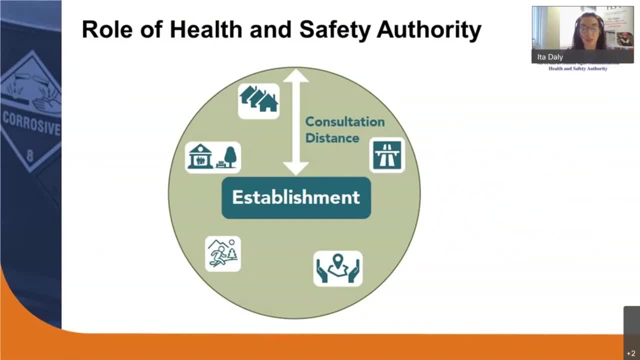 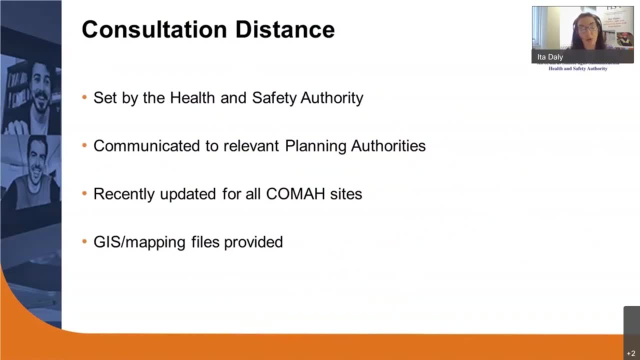 around each establishment, and this is called the consultation distance. Now, what do we mean by consultation distance? Well, in essence, it's a protective zone around a COMA establishment to ensure the risk to human health and the environment is minimized, especially for the developments I outlined already. 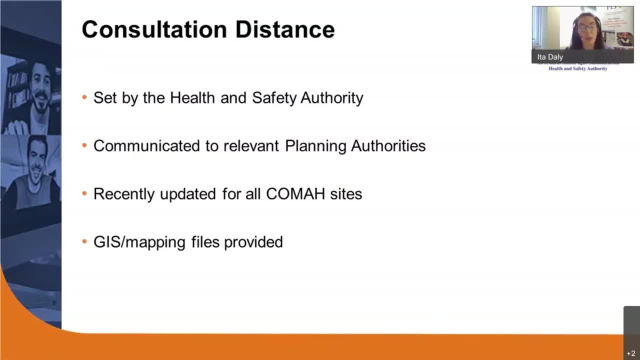 So residential areas, buildings and areas of public use, recreational areas and so on. And once this consultation distance is set for an establishment, it then must be formally communicated to all relevant planning bodies. In 2021, the consultation distances for all establishments were reviewed and updated. 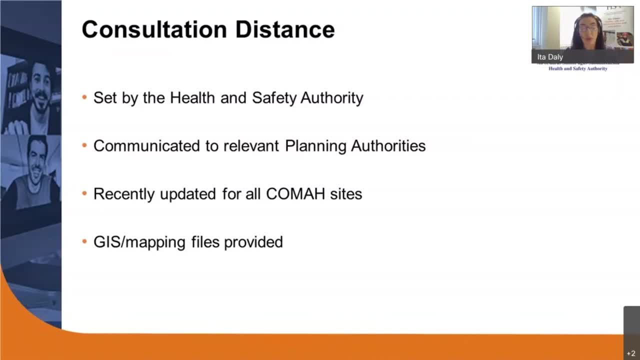 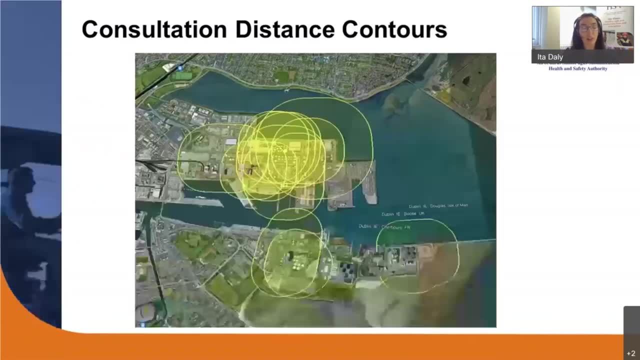 and details of the revised consultation distances were sent to the relevant planning authorities and to site operators in the form of a GIS file. So here is an example of what those mapping files look like overlaid in a map. This is an area with multiple COMA sites. 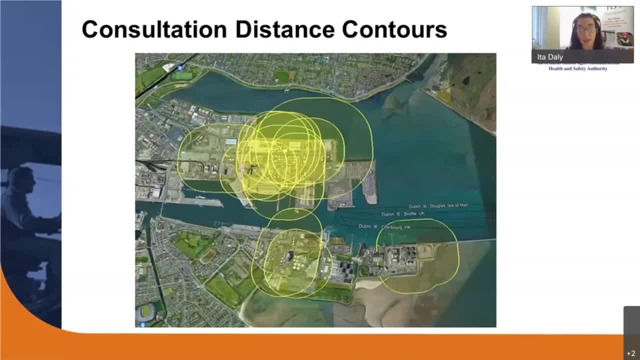 So the consultation distance is generated using the risk-based approach described in the new guidance document, and it corresponds to a one by 10 to the minus nine or one in a billion fatality risk contour. It is important to point out that this risk figure 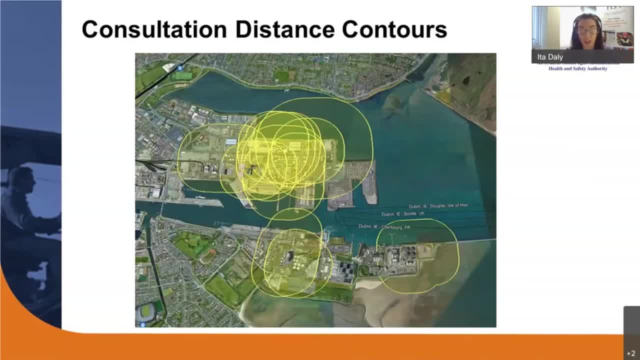 is based on the inventory provided in your COMA notification. Therefore, if there are modifications on a COMA site, including changes to the quantity of dangerous substances, it is vital that these modifications are communicated to the authority through the significant modification process Now, once a planning body have been informed. 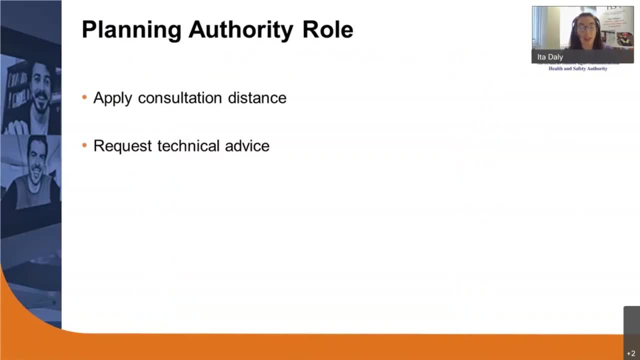 of the consultation distance around a site. they then, in turn, are required to seek technical advice from the HSA for certain types of proposed development within the consultation distance. These types of proposed development are set out in the planning and development regulations, and they range from the provision of housing. 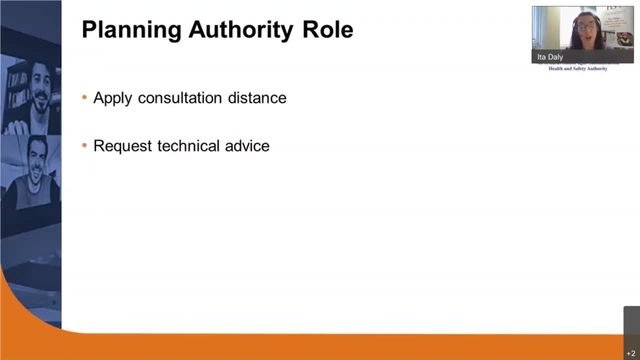 to schools, hospitals and creches, to commercial, industrial or office development for 20 or more employees, And as well as new developments. the requirement for technical advice also extends to new developments within the consultation distance development on a coma site or for permission for a new coma establishment. 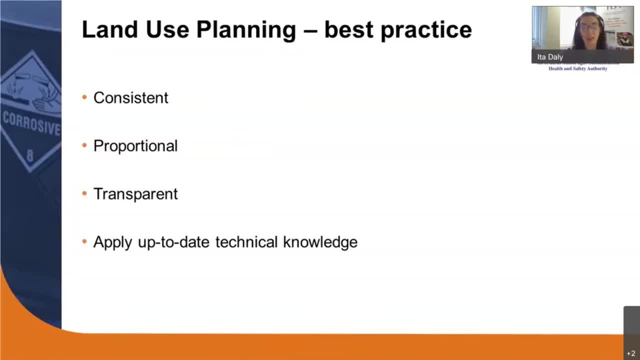 European best practice advises that a technical land use planning advice system should apply the principles of consistency, so the outcomes from broadly similar situations are broadly the same under similar conditions. proportionality, so again the constraint should be proportional to the level of risk. and lastly, transparency, so an understandable, clear and well-described. 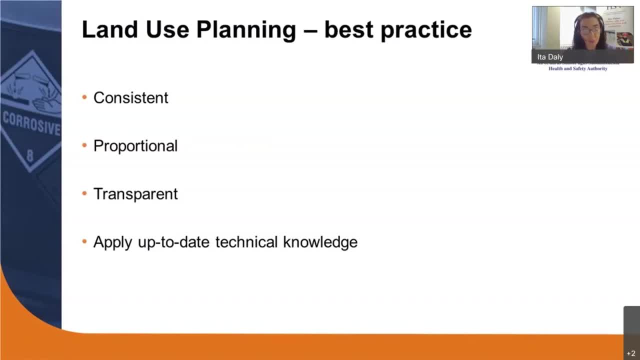 decision-making process should exist. Best practice also requires that account be taken of the most recent technical knowledge. The system set out in the new guidance document adheres to these principles and also takes account of recent publications at an EU level, along with taking account of any relevant technical knowledge. in the provision of technical 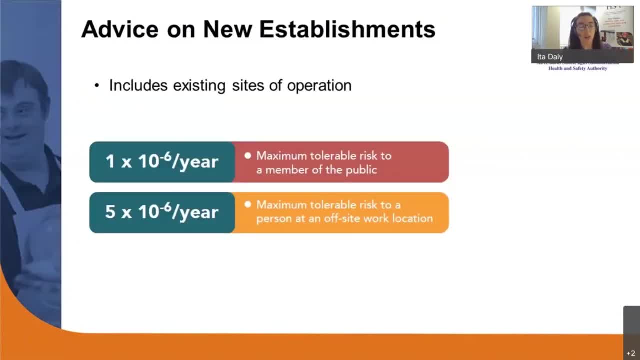 land use planning advice. So just to cover, now that we know the process around how land use planning is managed, I want to cover how the technical advice is managed. First let's look at new establishments. This covers the siting and development of newly constructed coma establishments. but 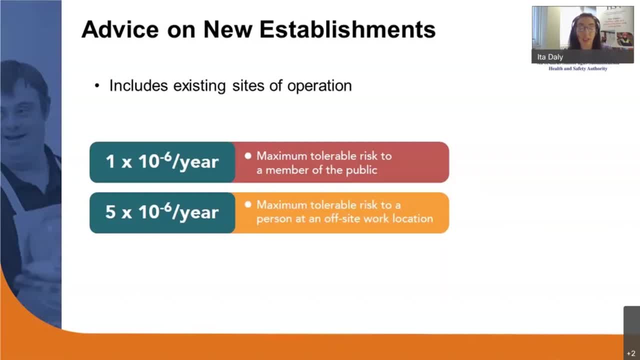 it also includes sites of existing operation where the coma regulations did not previously apply, but now such a site intends on increasing their inventory of dangerous substances above the coma thresholds and thereby bringing them within the scope of the coma regulations, In keeping with the longer-term aims for planning. there are a number of areas that need to be. 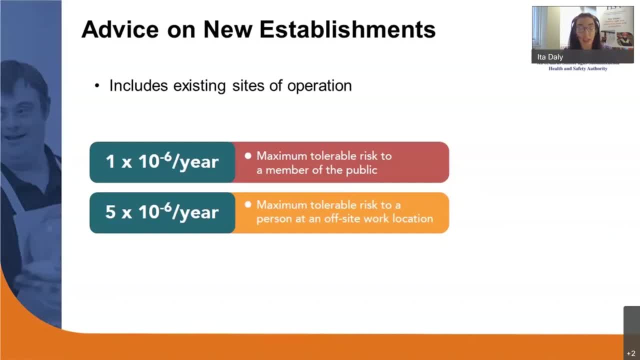 addressed, For example, land use planning. under the CIVASO directive, technical advice in relation to new coma establishments will be more stringent than that which applies to existing coma establishments. The individual location-based risk counters for new establishments not to be exceeded are set out here on the slide. 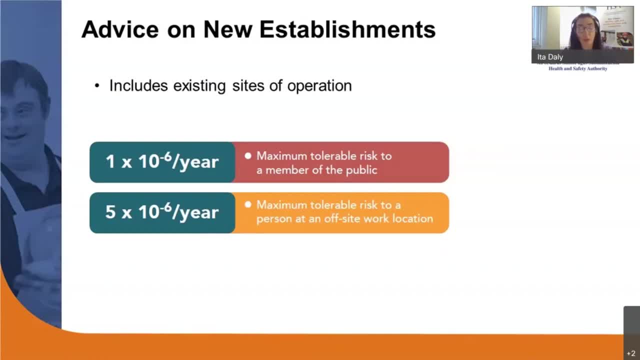 So you can see that the maximum tolerable risk to a member of the public should not exceed 1 by 10 to the minus 6 per year, and the maximum tolerable risk to a person at an off-site work location should not exceed 5 by 10 to the minus 6 per year. 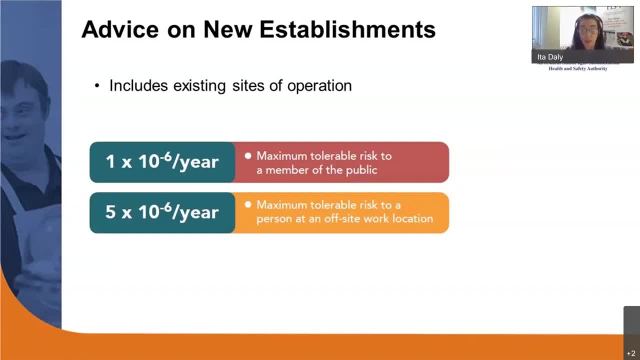 However, even if these individual risk criteria are met for a specific development, a societal risk evaluation may also be necessary. I'll cover societal risk in more detail in a moment. In addition, the advice given to planning bodies on a new establishment may also include 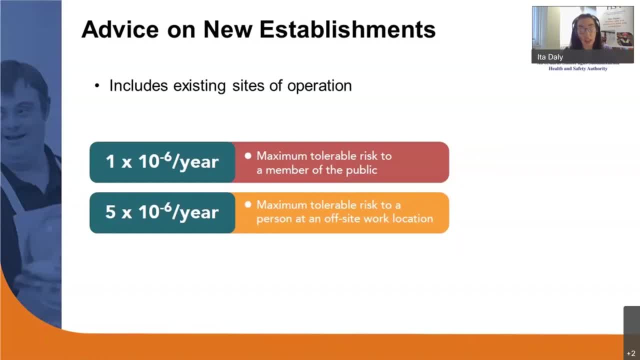 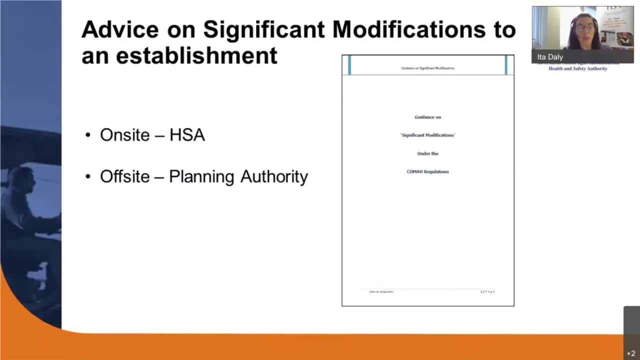 an advisory to consult with the principal response agencies in relation to emergency planning. So, moving on to advice on significant modifications to an establishment, As you are aware, the authority have already published guidance on significant modifications in 2019.. In summary, the HSA regulates the on-site risk element, setting limits for the tolerable. 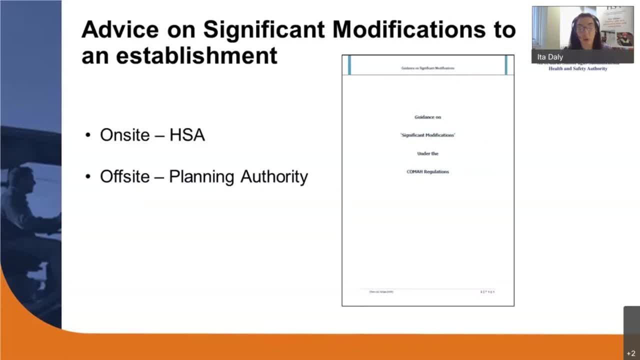 level of risk increase that will be permitted and then generally requiring the lowest level of increased risk through the use of additional technical measures. But for off-site risk, the referral trigger is an off-site location fatality risk equal to or greater than 1 by 10 to the minus 6 per year, and it will then be referred to the 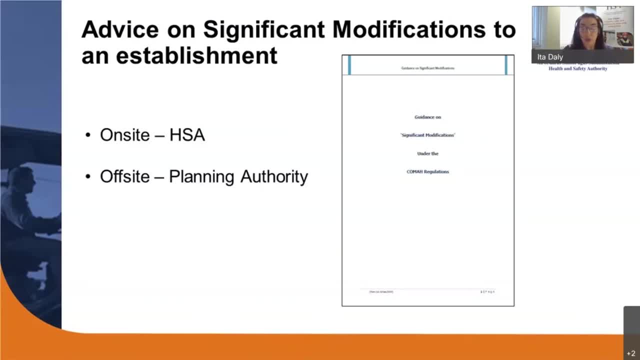 planning authority, The HSA, must always be notified by operators in advance of any planned significant modification, and the procedures outlined in the guidance on significant modifications under the COMA regulations must be followed, irrespective of whether or not a modification will be subject to a planning application. 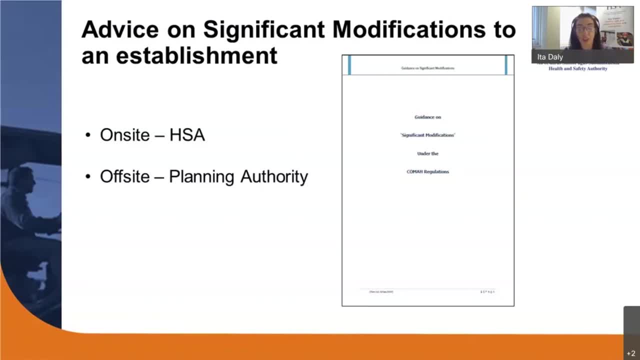 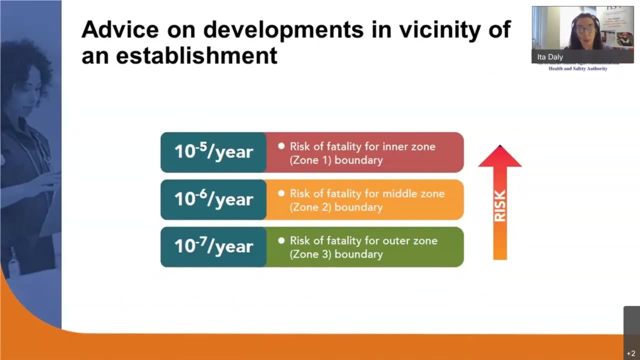 And we will use the data and documentation submitted in the significant modification process when providing technical advice to a planning authority For development. in the vicinity of an establishment which is within the consultation distance, three zones of risk are plotted around the establishment. These three zones are based on the location, quantity and hazards of the dangerous substances. 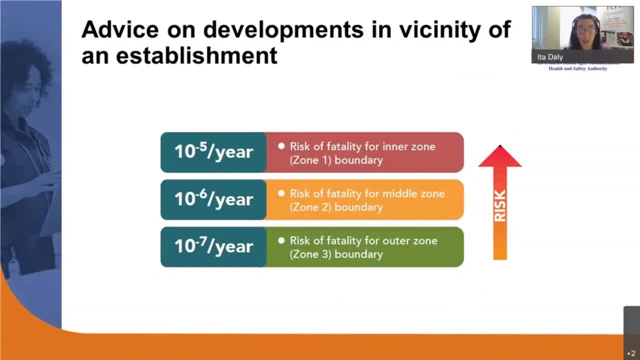 present on the COMA site, And this is based on the information submitted in your COMA notification. The zones are inner or zone 1, middle or zone 2, outer or zone 3, and you can see the risk figures for each of the zones, with the inner being the most restrictive at 1 by 10 to the 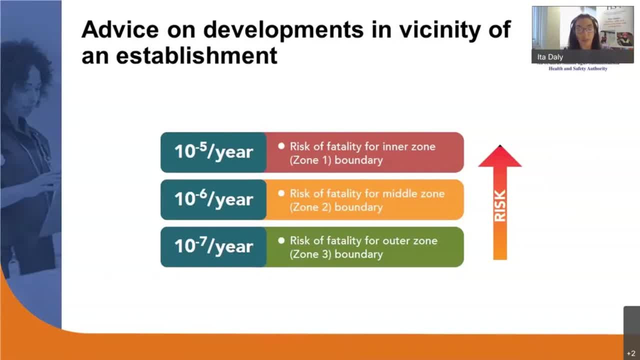 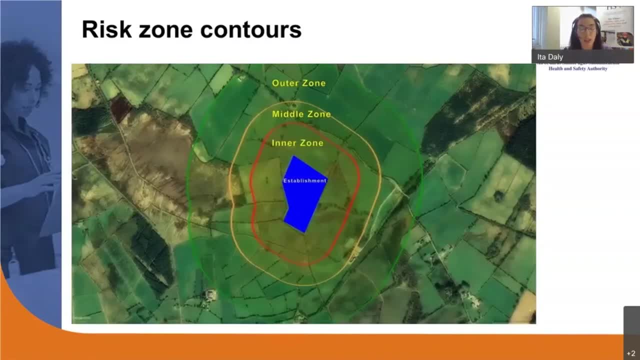 minus 5, extending to 1 by 10, to the minus 7 for the outer zone. To give you an idea of what these risk zones look like, here on the map is a fictitious COMA site With the three risk zones overlaid. 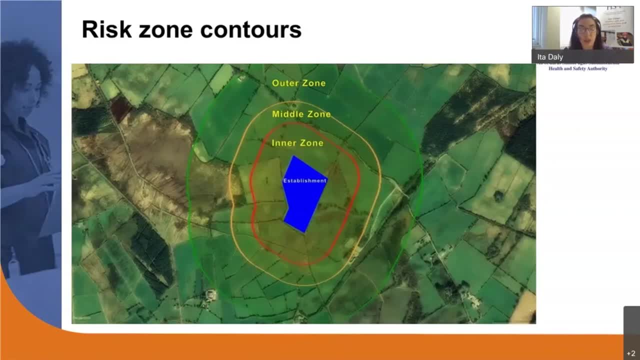 You can see that the inner zone with the red contour is the one closest to the site boundary And occasionally, depending on the nature and quantity of the dangerous substances, the inner zone may not extend outside the south boundary. The middle zone, then, is the sits outside. the inner is the is the orange contour and the. 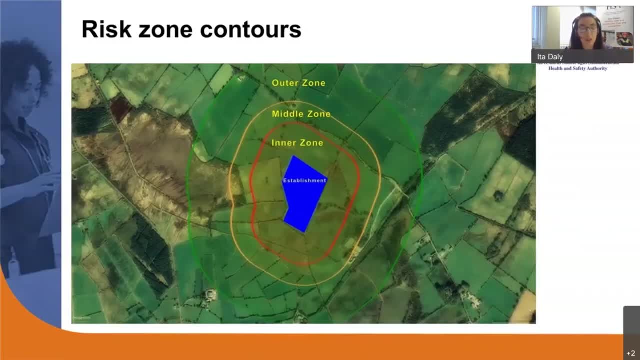 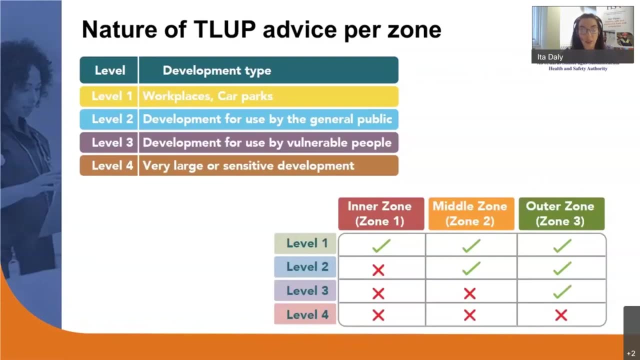 outer zone is the green contour. So associated with each of these three zones are four levels of development, And these levels are set out here in the top table on the left, with level one being the least sensitive, increasing to level four for very large or sensitive development. 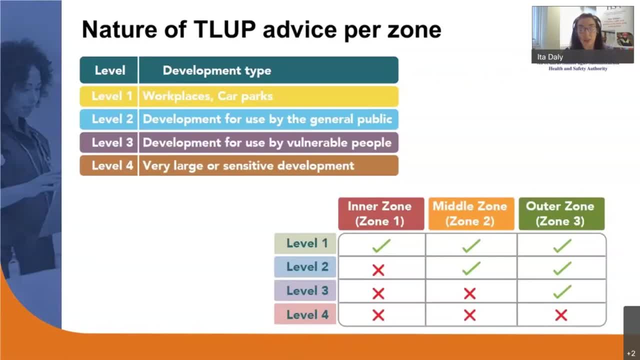 The full text of the development sensitivity levels are set out in appendix two of the new guidance document. But just to give you a general sense, level one covers people at work and parking areas. Level two is for development for use by the general public, such as housing, hotels and 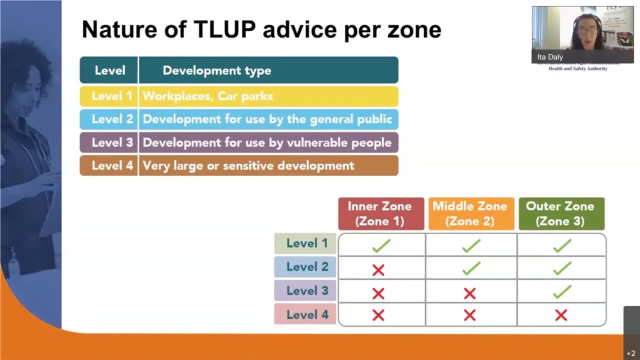 transport links. Level three covers development for use by vulnerable people, like hospitals, schools and creches, Sheltered housing, nursing homes, And level four, then, is for very large and sensitive developments, things like larger scale hospitals and education settings and very large outdoor public use spaces, such 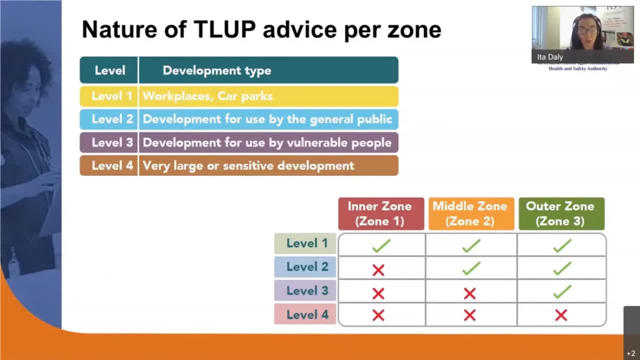 as theme parks, sports stadia and so on. So when the sensitivity level of the development has been determined, along with the location within either zone one, two or three, then the table on the bottom right of the slide here gives an indication of what the authority's advice would be. 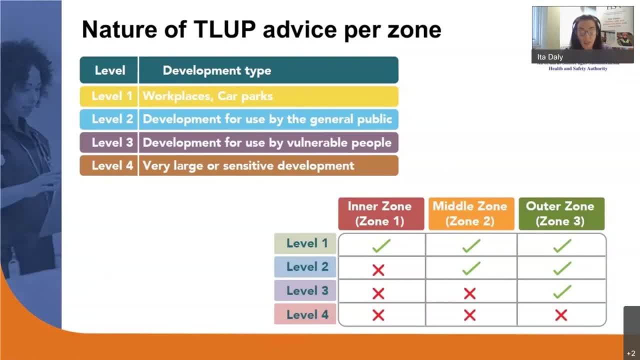 You can see that sensitivity level one development would not be advised against in any of the three zones, but sensitivity level four would be advised against in all three of the zones. So this system is based on individual risk. So that is the risk to a person permanently located outside the establishment. 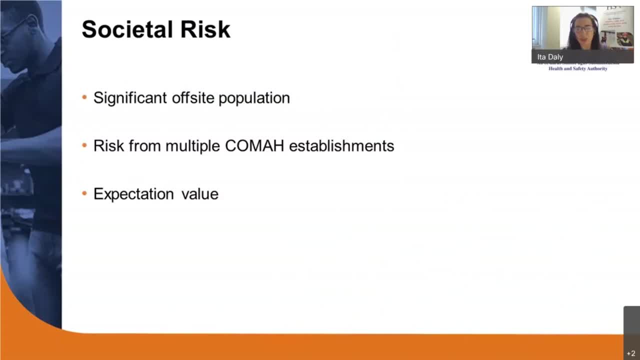 However, there are times where the risk of multiple fatalities from an accident or societal risk should be taken into account more explicitly. For example, this may include where a planning application relates to a proposed significant offsite development with significant population density or where there is already a significant 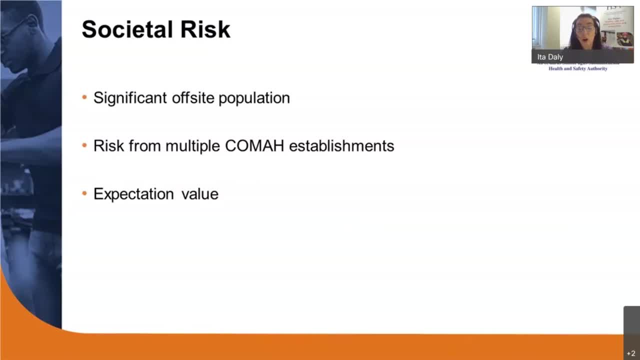 population residing or working within the risk zone or where the risk is emanating from more than one establishment. So to take account of societal risk in such situations, we will initially obtain an estimate of the expectation value, And the expectation value is a multiplication of accident frequency expressed in chances. 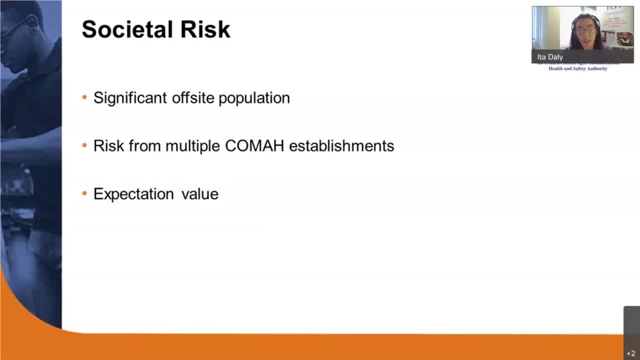 per million and the number of people suffering a fatality in that accident. Societal risk is covered in more detail in section 1.7 of the new guidance And in general the expectation value should not exceed 10,000.. If it does, the advice to the planning authority would be always to advise against the development. 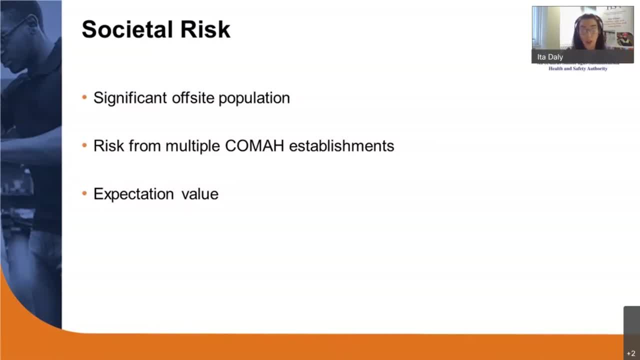 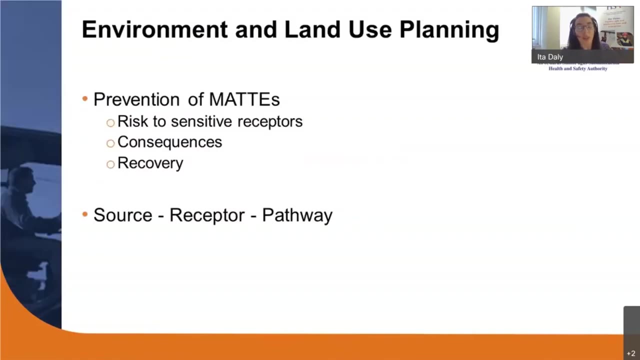 Especially large scale or sensitive development within the consultation distance will look much more important. For example, the envoy to the site of that site will require a spatial risk evaluation and the societal risk criterion is applied in addition to the individual risk criterion previously outlined. Just to touch on the environmental aspects in the context of land use planning, the prevention, 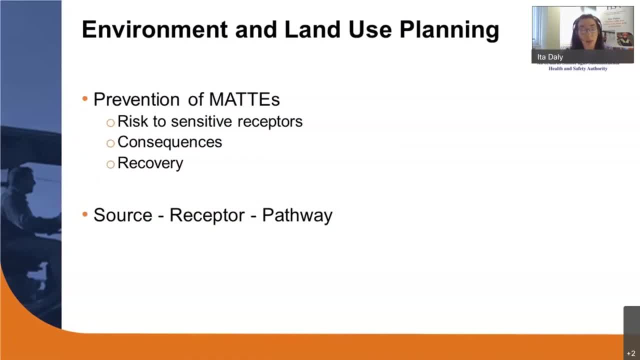 of maties will be the primary objective, and it is expected that accident pathways will be prevented. Where this is not practicable, or in the context of significant modifications at existing co-establishments, We will need to consider the marriages and who's doing what, and how the pieces will. 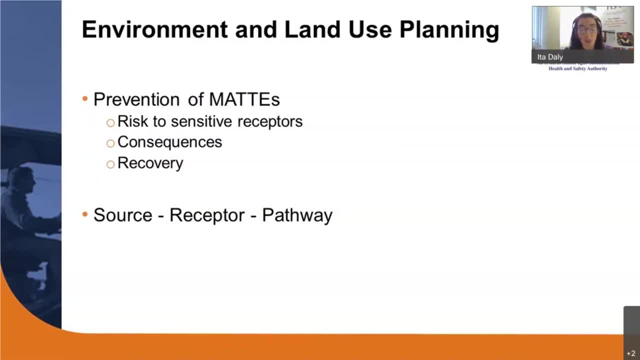 be used to the environment focuses on the specific risks to sensitive receptors within the local environment, the extent of consequences to such receptors and then the ability of such receptors to recover. so environmental damage may be relatively long lasting, but it is not necessarily irreversible. so the recovery of habitats within a reasonable period of time is possible and depending on the 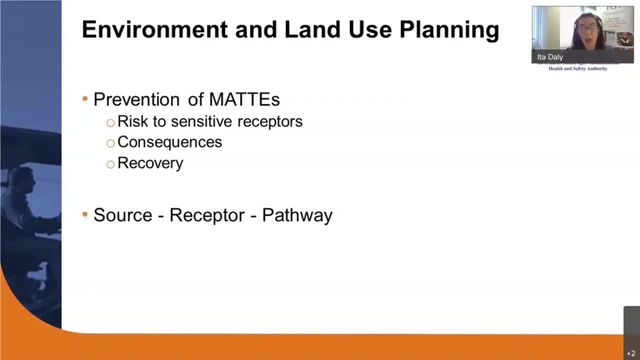 dangerous substance involved, and this information, then, can be weighed up from providing advice. the full detail relating to land use planning and the environment is contained within section 1.8 of the new guidance document, just to touch on the public information zone. so, prior to the coma regulations of 2015, the specified area was defined as an area at greater risk of being. 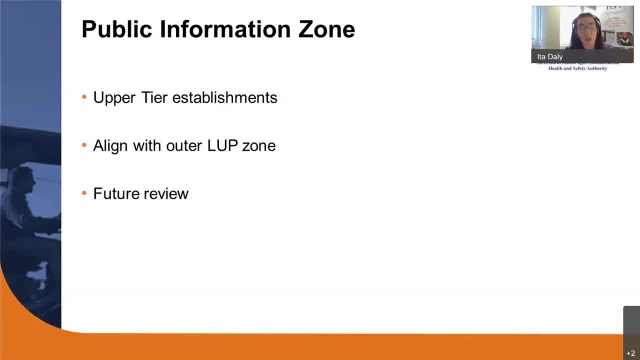 affected by a major accident and within which an upper tier establishment had to supply information directly to persons in in that area on the appropriate action to take in an emergency. so, whilst this area still exists, it is no longer referred to as the specified area. the requirement is to provide this information. the requirement to provide this information still. 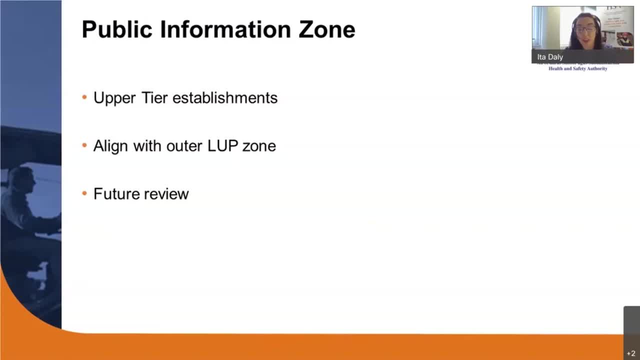 applies under the 2015 coma regulations, but this area is now to be known as the public information zone, so this zone will, at a minimum, coincide with the outer land use planning zone, and the hsa will use its discretion as to whether it should be enlarged further, based on the consequences of the 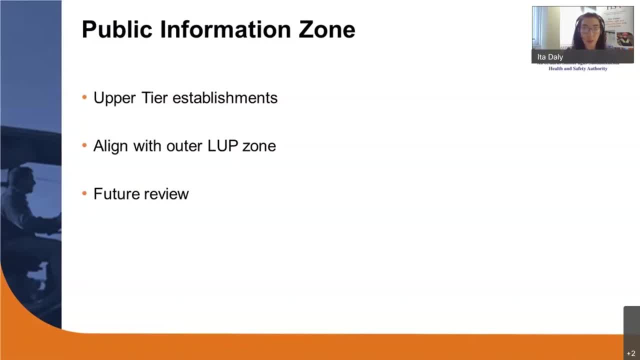 previous year's plan. so the current plan is to make sure that the area is used as a public information zone until they are replaced, which will happen as generic land use planning advice for each establishment is rolled out to planning authorities. and that leads me on to my last slide. 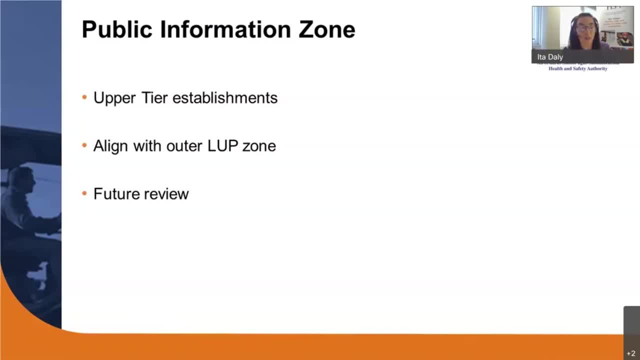 now covering the development of such generic advice. so the authority plans on preparing generic land use planning advice for all coma establishments? uh, this generic advice will be based on the data provided in your coma notification and will include development of the three risk contours for inner, middle and outer zones i described earlier. once completed this generic 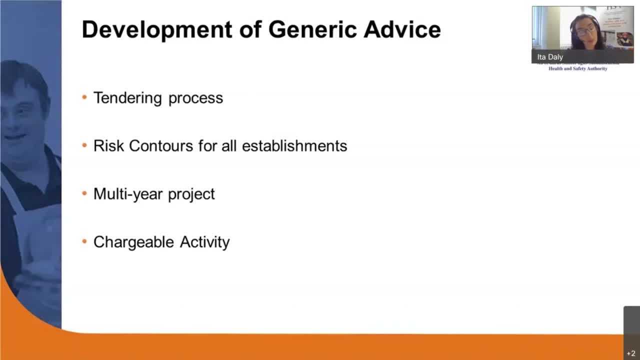 advice will then be provided to the relevant planning bodies. um due to the nature and volume of the task, the authority is seeking external technical expertise to develop this advice for each establishment, subject to the regulations. the tender process is ongoing and we don't really have a timeline as to when the work will commence as yet, but it will be a multi-year. 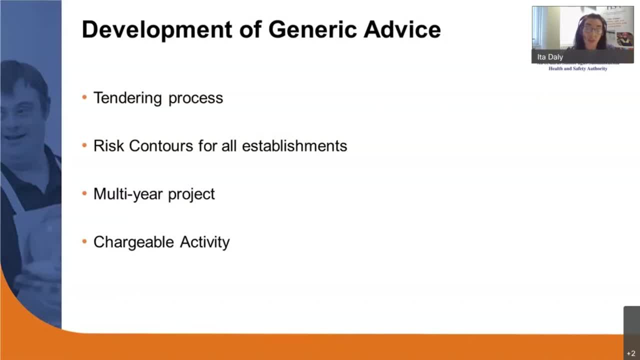 project. the charging of fees for services under coma is covered by regulation 27 of the coma regulations and it sets out the activities for which the authority may charge fees and one of those is the provision of technical land use planning advice. so this will be a chargeable. 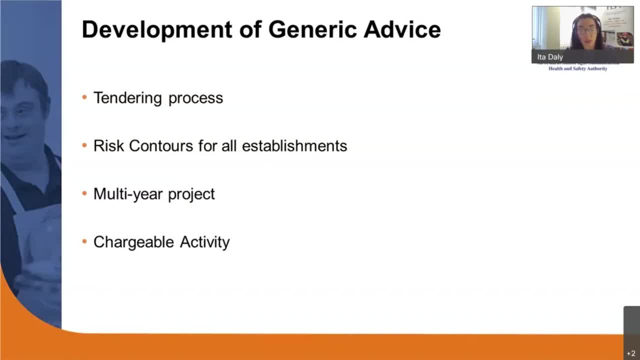 activity and as set out in the scale of fees of january 1st 2016, the initial fee will be 3 000 euro covering the first five days, up to a maximum of 20 days, at 600 euro additional per day, and further information on charging is available on the coma pages um of the authority's website. 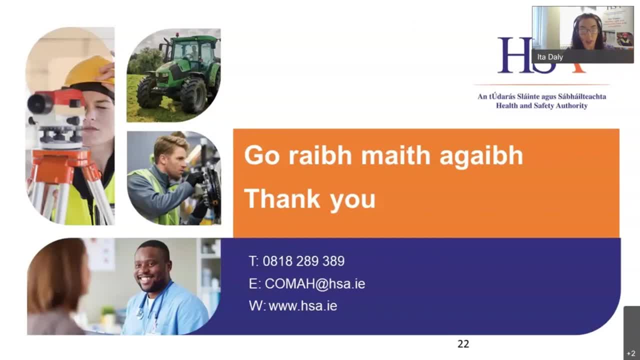 so that brings me to the end of my section. so for now, i'm going to hand you over to pat and he's going to take you through some of the more technical elements of the new guidance document. thanks pat, thanks isa, hello and uh, welcome to the second part of the webinar, and i'm going to deal with parts two and three of 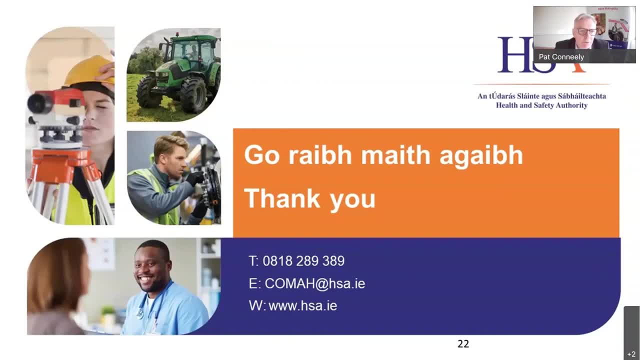 our new guidance on technical land- just planning advice- which we just launched, in january of this year. um, i'm pat kneely. i'm head of the coma unit, which is responsibility in this area, and, as isa mentioned, it's uh, if you have questions, it's probably best to hold them to the end, certainly. 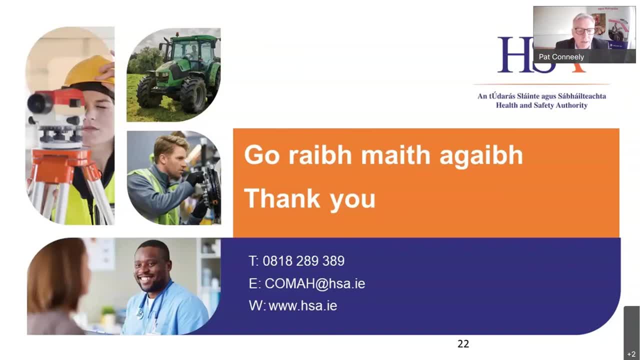 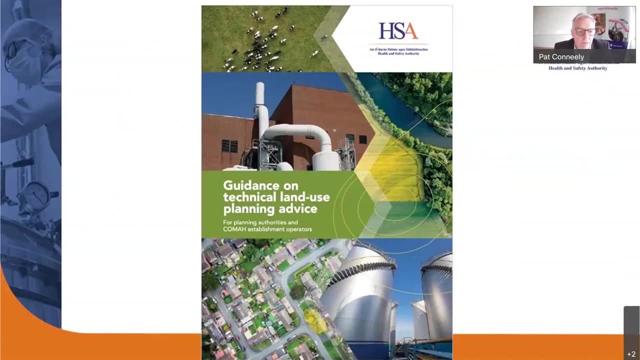 make a note of them, but we'll try and deal with them at the end and if um, perhaps even you'll find um your question has been answered before we get to the end. so hopefully that will be the case. okay, so there we go, um, so the guidance sets out in considerable detail how the authority will. 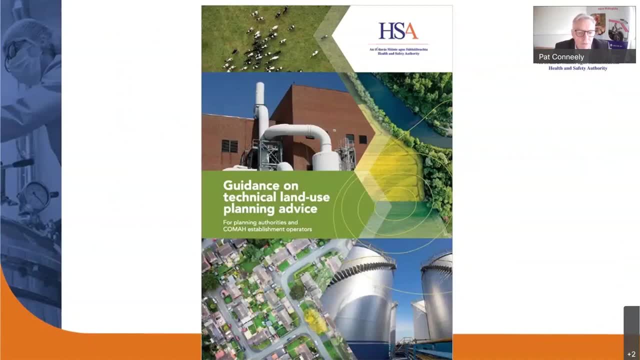 develop generic advice for planning authorities around coma establishments and, as he said, we intentionally want that over the next few years. um, the guidance also contains advice for planners on how to interpret that technical guidance and we covered that in a previous webinar. so if you're in that aspect of it, you should look that up. 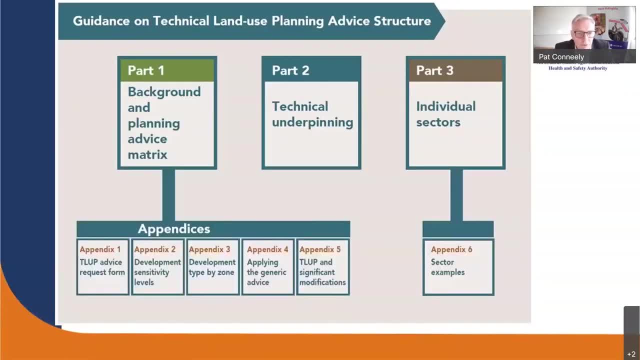 now um isa has brought you through part one of the guidance, and i will now give you an overview of parts two and three, and i'll particularly emphasize and highlight where we have made changes. parts two and three are quite technical. part two sets out the technical underpinning of the method. 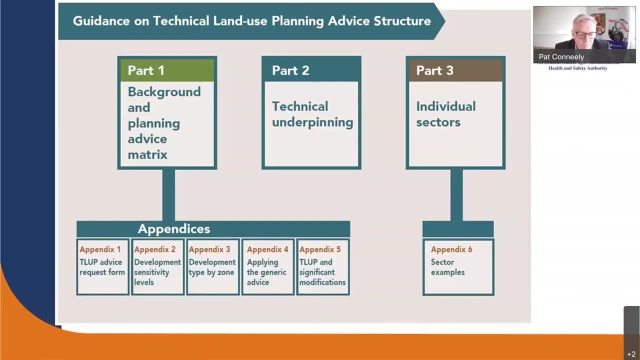 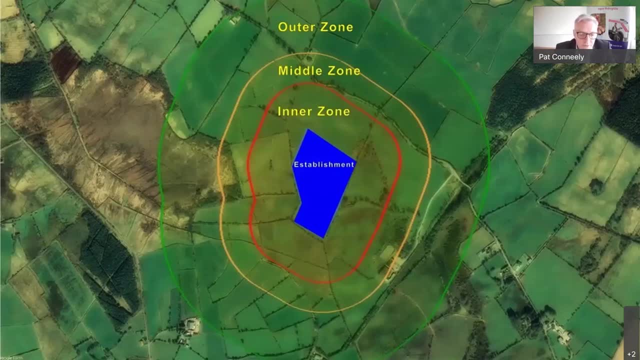 while part three describes how it will be applied in the different sectors. of course, again reiterating what isa has said, the ultimate aim of all this is to provide three generic advice contours around each coma establishment and that will be supplied to the planning authorities and they can use that then for the future control of development around those sites. 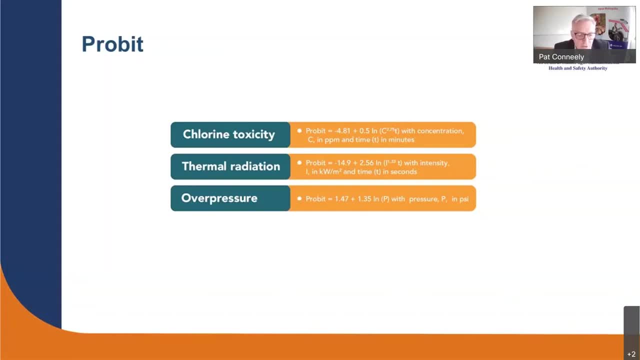 now, a key element of the approach is the estimation of the consequences of exposure to a hazardous agent. the method employed relies on the use of probit equations to address this question, and here are three probit equations. the first is for chlorine toxicity, and the probit provides a 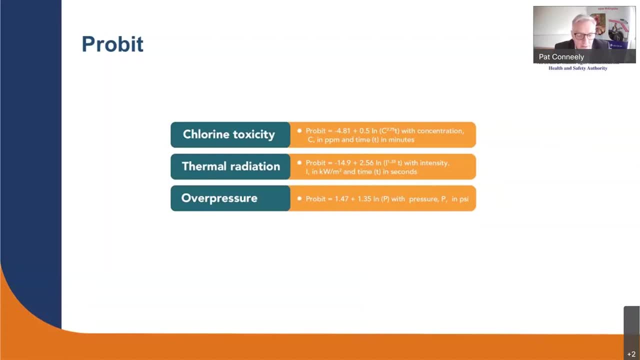 lethality value for exposure to chlorine gas and it depends on the exposure concentration, which is c in the equation and t, the exposure time in minutes. and, as you can see in that equation, the concentration has a big impact on the probit value. the second probit is for fatality from. 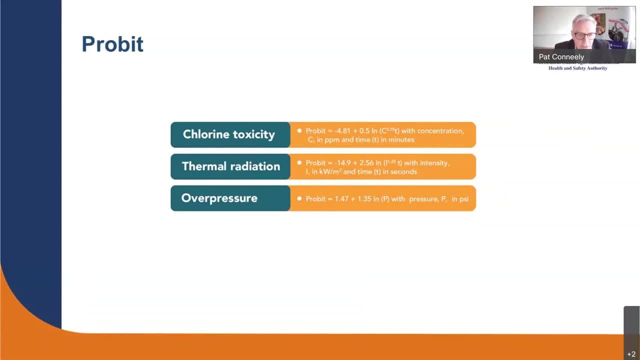 exposure to terminal radiation by i, and the duration of exposure, which in this equation is in seconds, is represented by t. the final problem is for fatality from overpressure. here the value depends only on the intensity of the overpressure, and there is no time effect on that. 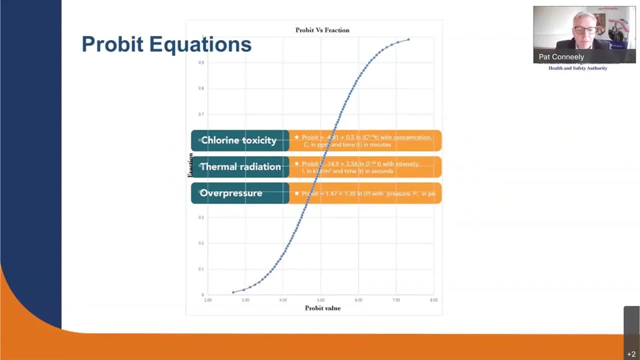 so the utility of these probit functions and values is that we can obtain, from specific exposure scenarios, we can obtain values that can be translated to fraction of fatality experienced in exposed population, and this is really useful when trying to convert estimated exposure consequences to a risk of fatality, which is required to generate. 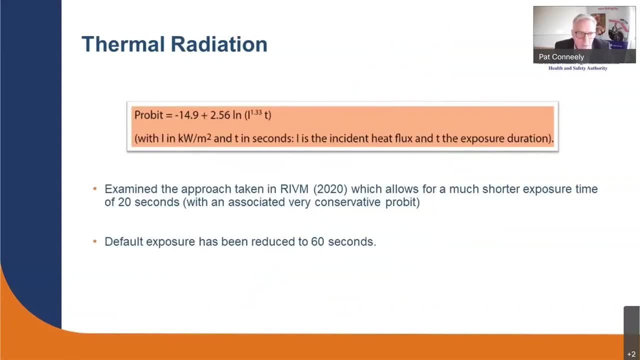 the largest planning risk contours. the probit for use for thermal radiation effects on people was derived by eisenberg in 1975.. most of the probits used in the method have been obtained from the dutch national institute of public information and the environment, and that's. 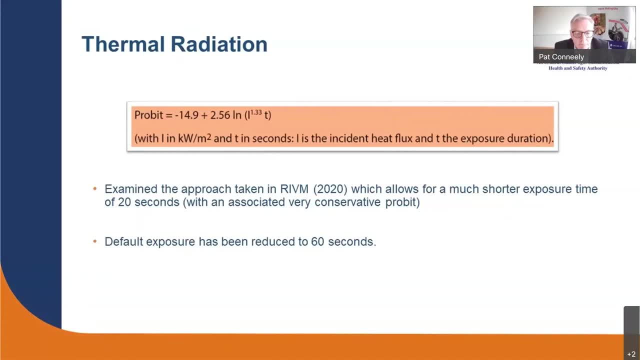 rivn for short in dutch, and that's the manual of bevy risk assessments. bevy refers to public safety of establishments decree, so it's similar to our own coma regulations and describes the approach to such risk assessments in the netherlands and we have drawn heavily on that for our own guidance, as we have on the approach. 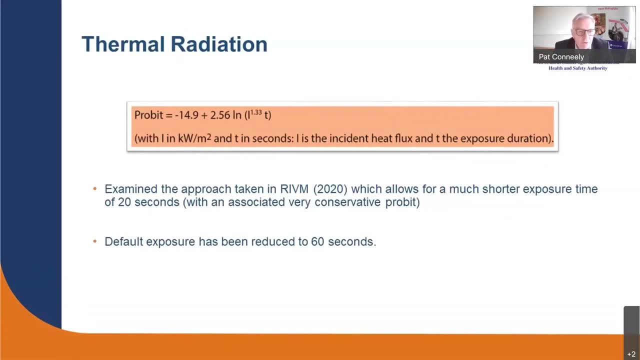 of the uk hse, particularly in relation to the matrix of advice and in developing our overall method. so one of the more notable changes that we've made in the revised guidance is to change the standard exposure time to pooled fire radiation from 75 seconds down to 60 seconds. 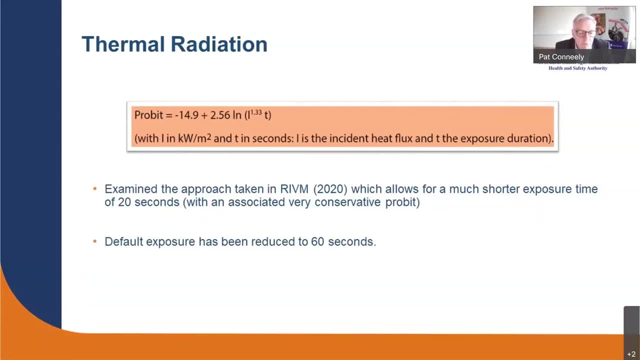 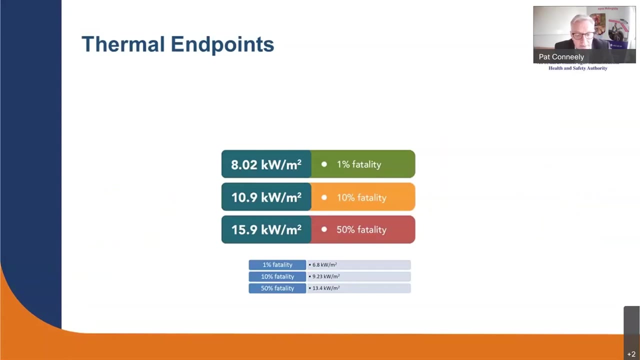 the same problem is used as was previously used, but the assumed exposure time has been reduced. the previous exposure time was considered to be overly conservative when compared with what the uk hse and the dutch approaches. well, that does have knock-on effects on the levels that might be used for consequence modeling, as shown here, because they have increased sufferiness. 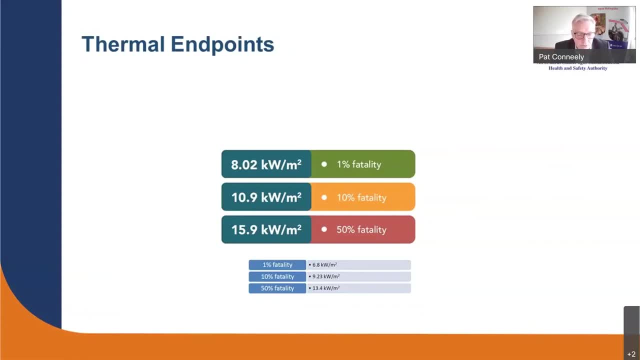 So 1%. it's from 6.8 kilowatts per meter squared up to 8.. For 10% it goes up to 10.9.. And for 50% it goes to 15.9.. Of course, thermal effects are mitigated. 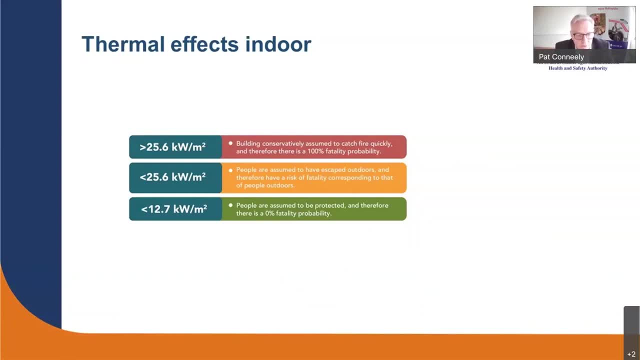 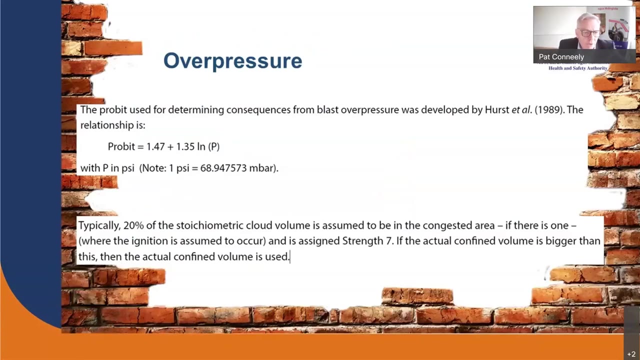 by the shielding effects of being within a building separated from the source. The values used in that context are unchanged from the previous version And generally exposure duration is not an issue for these endpoints. So if I go to look at overpressure now and the probit for that, we can see 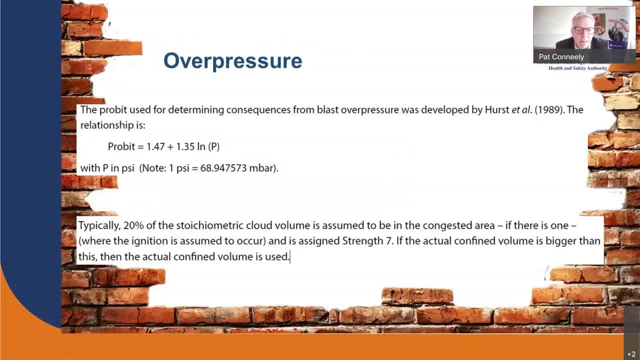 that when it comes to overpressure from explosive events, the approach is the same as in the previous version and the same probit is used For vapor cloud explosions, or VCEs. the standard model makes the assumption that 20% of the stoichiometric cloud volume 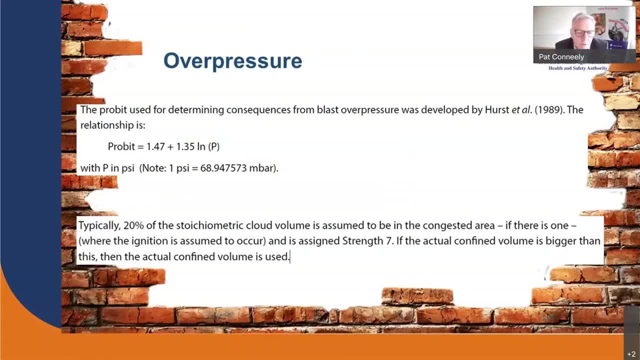 is in the confined area, And that's provided there is some confinement present. If the confined volume is known to be greater than that of the overpressure, then the overpressure volume is used and it will be modeled at strength seven using the TNO method, while the remaining unconfined cloud will 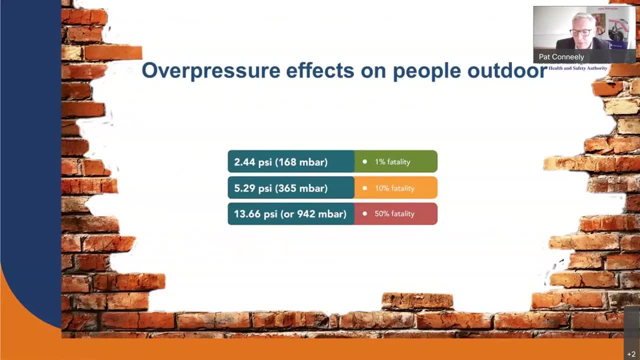 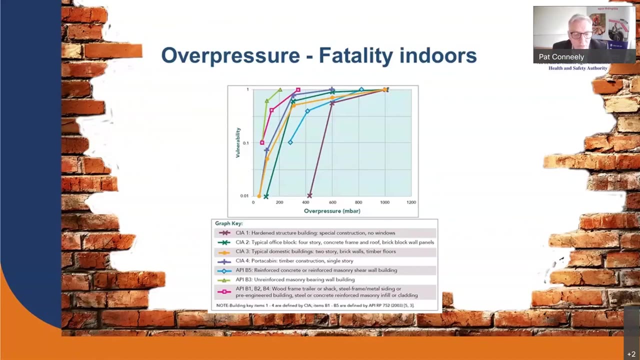 be modeled at strength two. So here are some landmark overpressure levels with associated fatality levels, And they're all unchanged from the previous version. When it comes to protection or lack of afforded by buildings, the chemical indices association approach is followed as it was in the previous version. 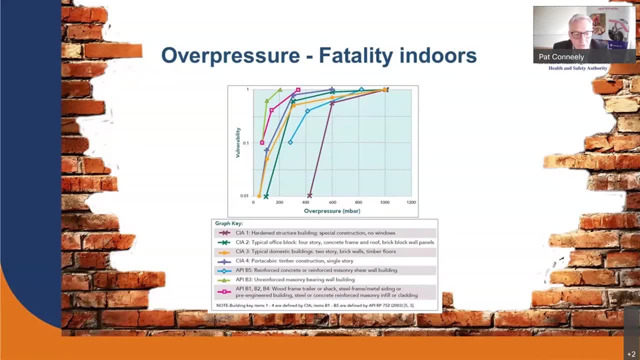 For residential buildings. the value from CIA curve three is used to derive fatality levels within buildings. The graph included in the guidance also includes curves in the American Petroleum Institute. So the methodology there is to look up the overpressure along the x-axis and up to the point it hits the curve. 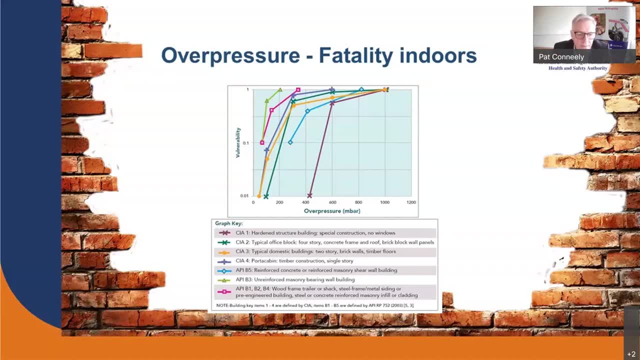 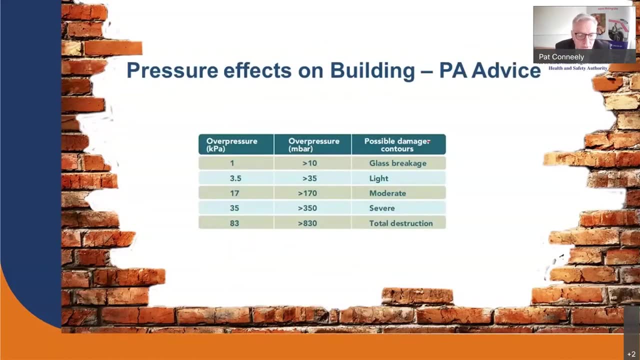 and then to go across and meet the fatality fraction on the y-axis. It is also intended to provide some consequence advice to planning authorities, along with the risk contours that are provided in the generic advice. So for damage to buildings from overpressure. 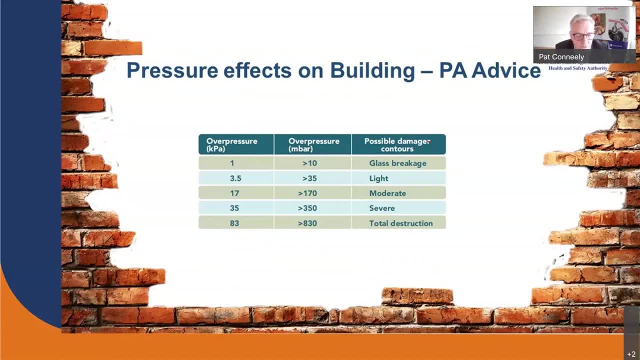 some of these contours could be included, most likely for glass breakage or light to moderate damage, for very unlikely- and therefore they'd be outside the standard contours, but still possible accidents. Because it's important, we feel, that the planning authorities are fully apprised of the contours. 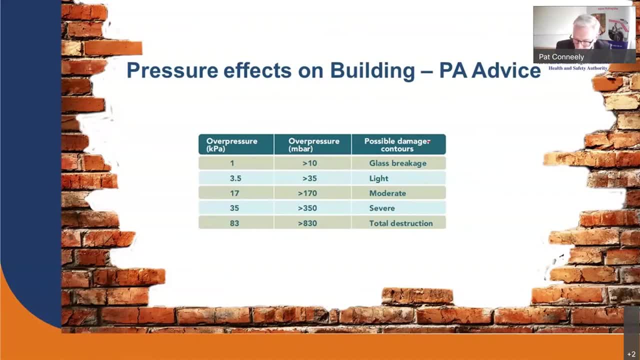 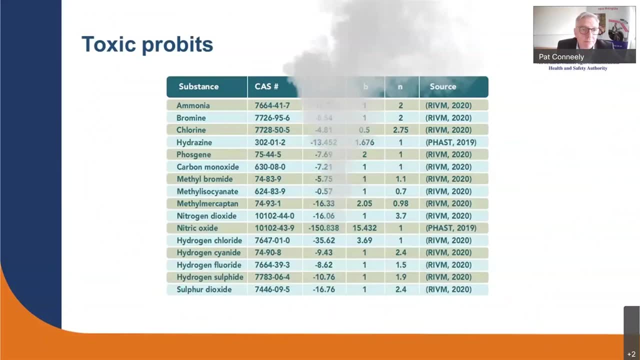 and of the consequences of the major accidents, as well as the risk. So an updated table of phobets has been included in the guidance. As you can see, most are from the Dutch publications that I previously referenced. A couple are also included there from FAST. 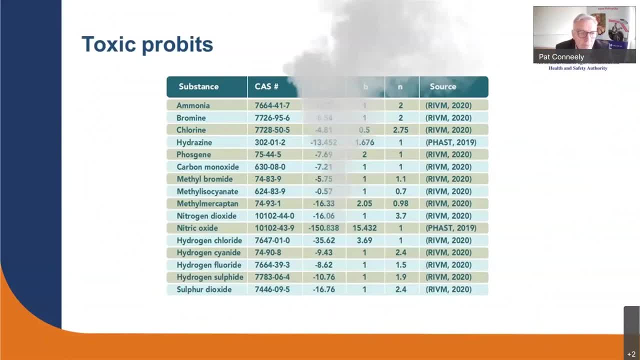 and those came from our expert group, And that gives me an opportunity to thank the expert group for sharing their knowledge and time and providing input in the earlier stages of the development of the guidance And, of course, in that context, the guidance. 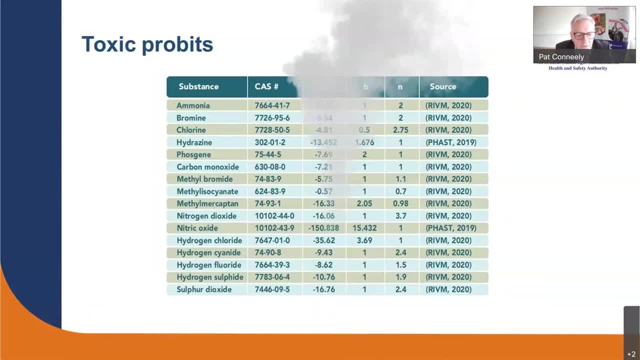 the draft guidance went out to public consultation earlier in 2021, and we received a lot of constructive feedback at that point and most of which we have tried to incorporate into the guidance, but more on that later. Now part two of the guidance also. 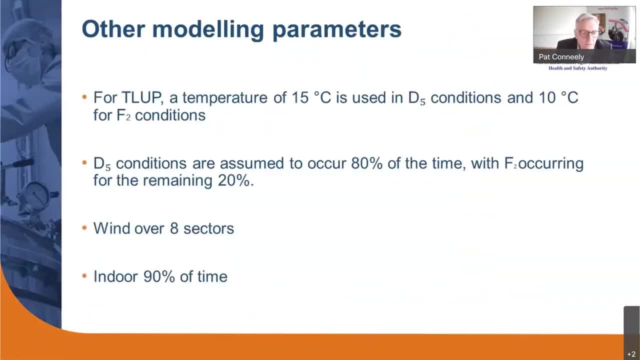 contains some other important modeling parameters to be used in the standard model. Modeling parameters are important because they are important to the development of the model, And they are important to the development of the model And they are important to the development of the model. 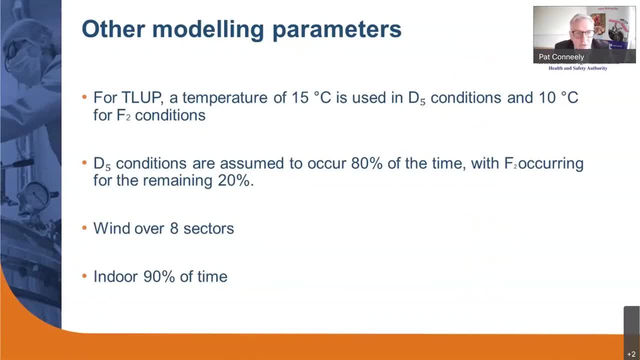 Modeling temperatures are now specified at 15 degrees for daytime conditions and 10 degrees for nighttime conditions, so that's new. Atmospheric stability conditions are specified as D5 for 80% of the time and F2 for the remaining 20%, so that's as before. 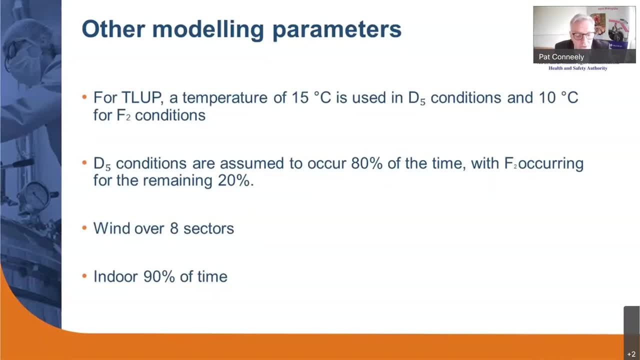 Wind direction is accounted for by taking account of the nearest weather station and using an eight sector probability fraction. In the standard model, receptors are assumed to be indoor for 90% of the time, so 10% outdoors, As before being indoors will in most situations. 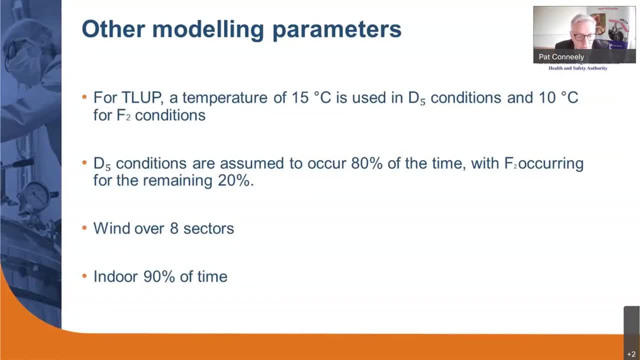 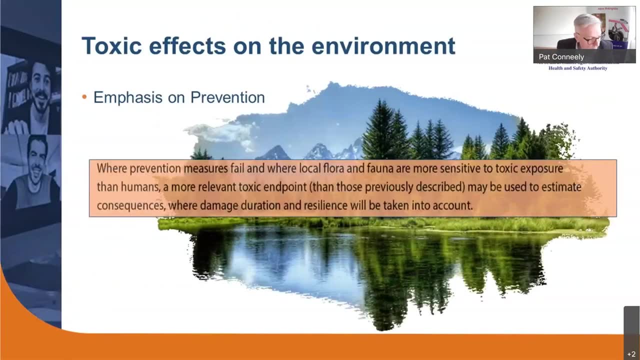 offer protection. Local terrain will also be accounted for with the surface roughness of 0.1 used by default. So in the provision of land use planning contours, environmental effects are actually not usually relevant, certainly not for existing establishments In relation to the siting of new establishments. 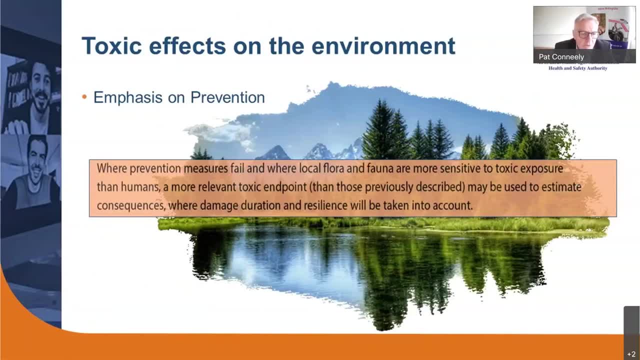 concerning the environment, the emphasis is always on prevention and the use of measures, usually around containment, but separation distances could also be relevant In this context. the toxic endpoints for humans may be sufficient, but sometimes a more sensitive endpoint may be necessary. 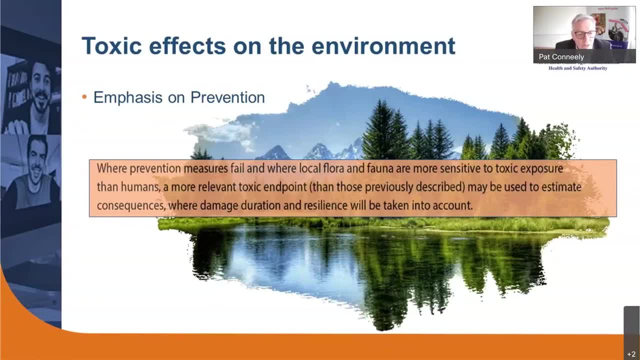 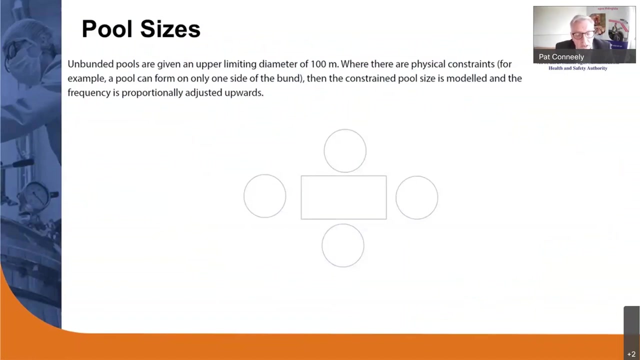 The choice of endpoint will depend on the data that may be available, and sometimes surrogates would have to be employed When examining environmental context, damage and consequences. in this context, damage duration and receptor resilience are also factored in. In modeling, pool size is also an important factor. 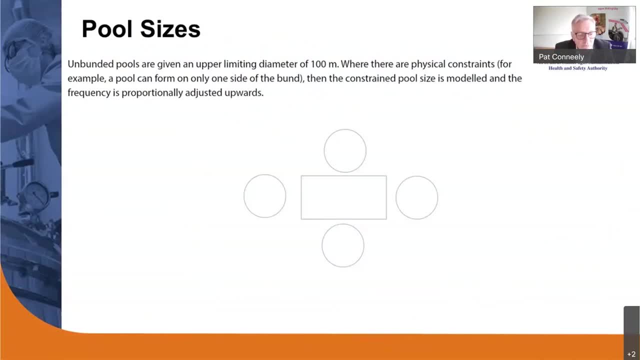 because these will influence the evaporation rate and also for flame height calculations for pool fires. The maximum diameter used for a pool will be 100 meters, provided that area is available. If physical restrictions mean that only a smaller size is possible, then that will be used. 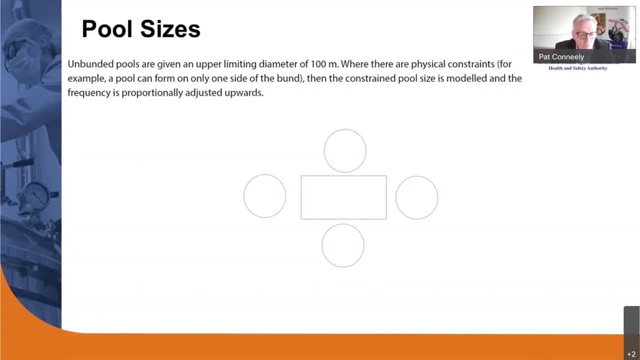 Another point I should make here is that bund overtopping pools may not always be possible due to a lack of space And, as you can see there in the second drawing out there, a pool cannot form on one side due to the presence of some sort of building or a wall. 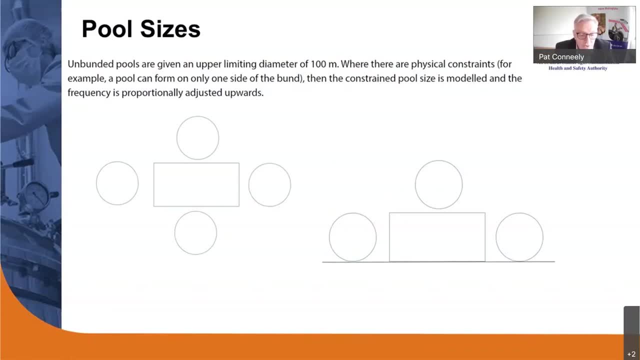 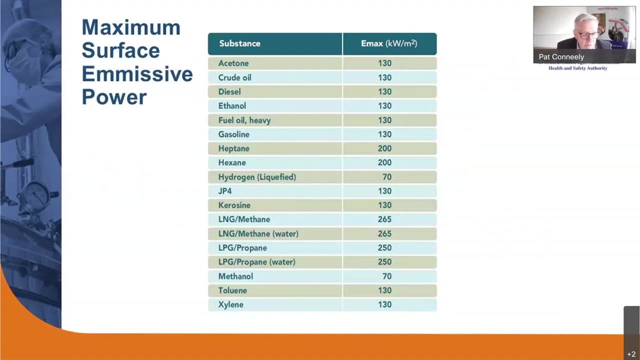 And in these circumstances the probability of an overtopping pool is just distributed over three pool locations instead of four, So each of the three become a little more probable, but there are only three locations For the modeling. a fresh approach has been taken for estimating thermal radiation. 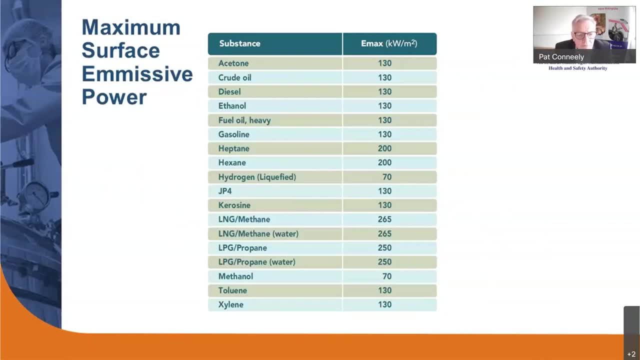 from pool fires. In the 2010 document, values for surface emission power of flames for surrogate class 1 and class 2 flammable liquids have been included. The current guidance does not include those, so that's an important change. It does include a table of maximum surface emission powers. 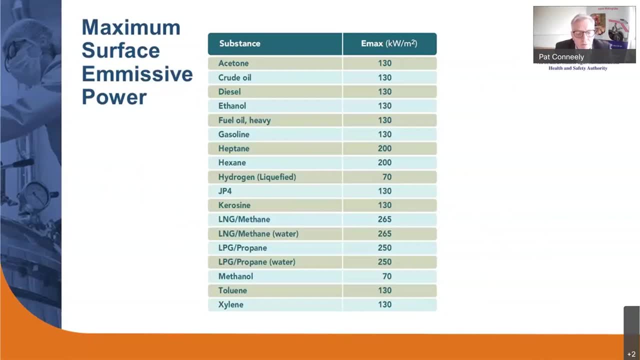 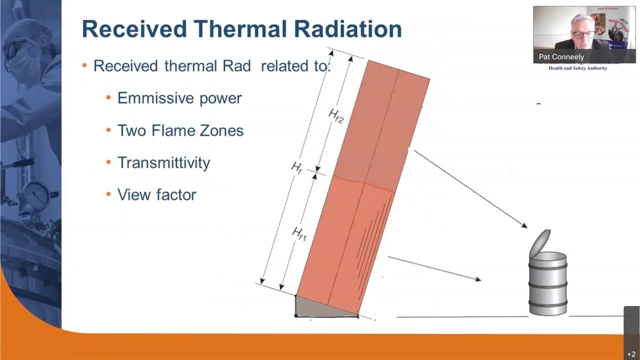 for a variety of common flammable liquids. However, The values are maximum values and some attenuation is necessary. when estimating the flux experience at a receptor, The preferred standard consequence model approach is to use a two zone flame model to take account of smoke obscuration, which typically 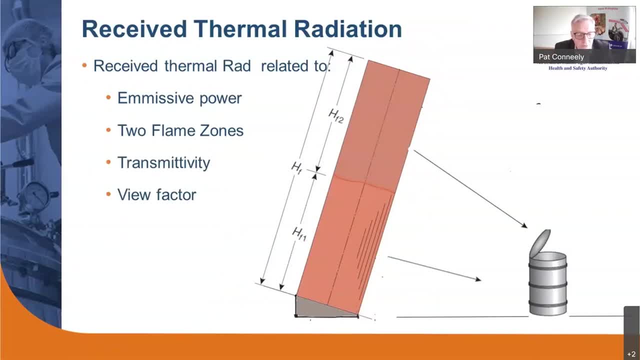 occurs in an upper zone. The distance to the receptor and the view factor to each flame zone is taken into account, as is the atmospheric transmittance. So this will yield a more realistic thermal radiation level, Which would be calculated on a case by case basis. 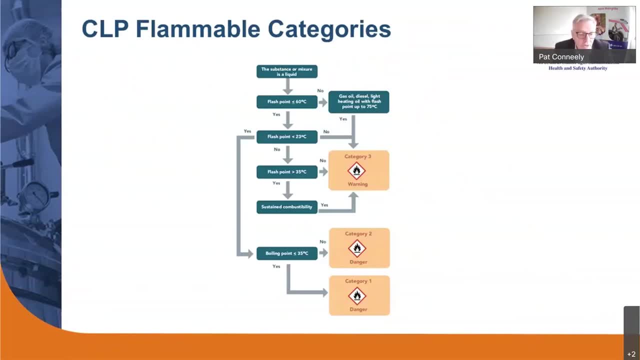 Flammable liquid classification now follows the classification, packaging and labeling regulation approach And a bridge graphic from ECHA's CLP guidance is included in our guidance so that the clear links between flash point and boiling point and flammable classification are clear. 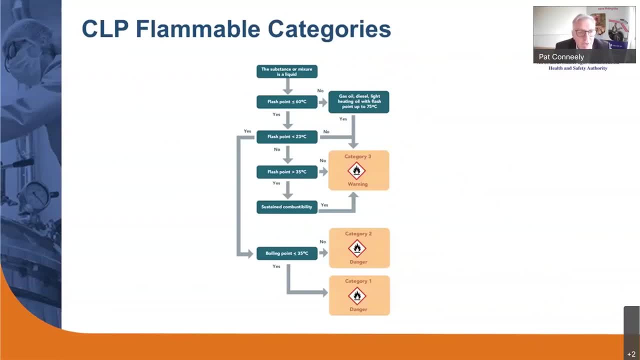 But, as I say, it's flammable liquid categories 1,, 2, and 3 that are found here. Now, in our experience, flammable liquid categories 1,, 2, and 3 are clear, But, as I say, it's flammable liquid categories 1,, 2,. and 3 that are found here Now in our experience. flammable liquid categories 1,, 2, and 3 that are found here Now in our experience. flammable liquid categories 1,, 2, and 3 that are found here. 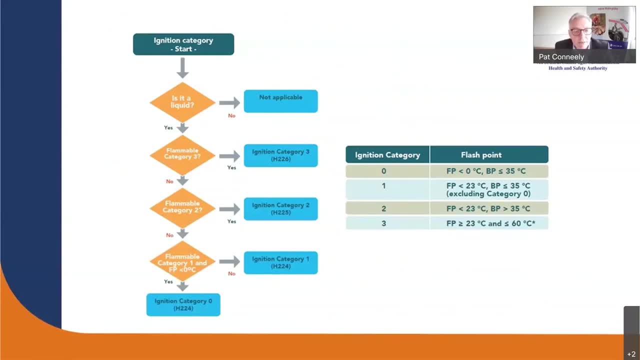 Again our guidance. ignition probability has been the source of dispute in London's planning advice area and contention Burgach, welcome to the veryск. so the guidance includes ignition probabilities for use in the standard model, So zero to three, shown in this graphic Two interpretation". 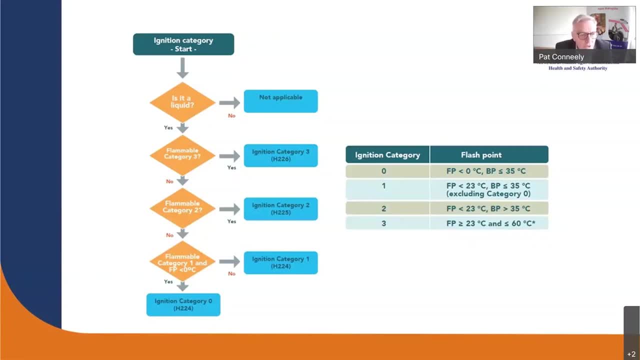 So for flammable categories 3, and for 2 that's relatively straightforward: Straight forward mapping, forward mapping. But for flammable category one there's a subdivision there into two ignition categories, and the substances that have the lowest flash point go into an ignition. 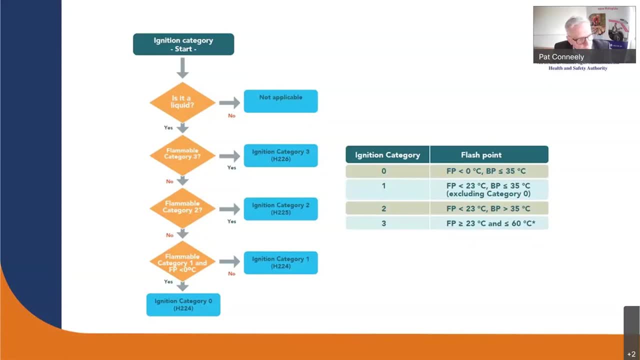 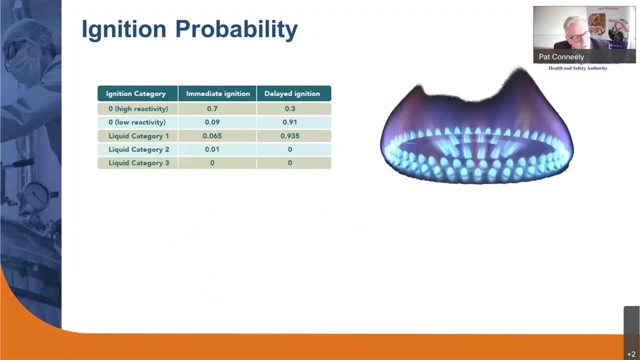 category zero. So this leads on to the assignment of ignition probabilities And, as you can see from this table, ignition is assumed to be either immediate or delayed. Class zero. high reactivity refers to the most flammable of gases. Class zero. 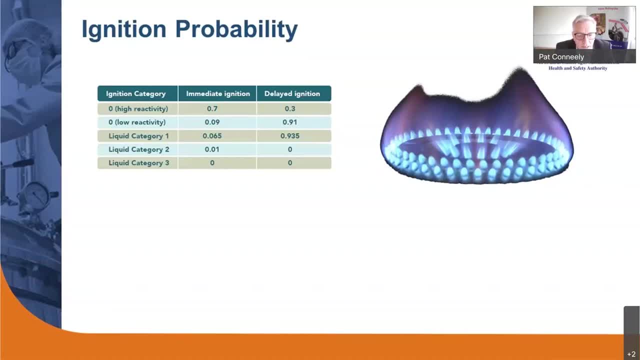 low reactivity refers to gases like methane and also is being used for ignition zero and flammable liquids. And then we have the other flammable liquids as shown, And by the time we get down to category three flammable liquids. it means that the 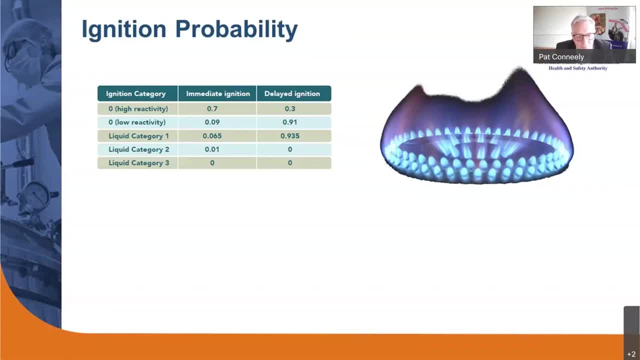 ignition probability is zero. So this is quite a change from the methodology that was in the previous version of the guidance and allows a lot more discrimination in relation to the type of flammable liquids that are stored on the site, And we've also included values that specifically 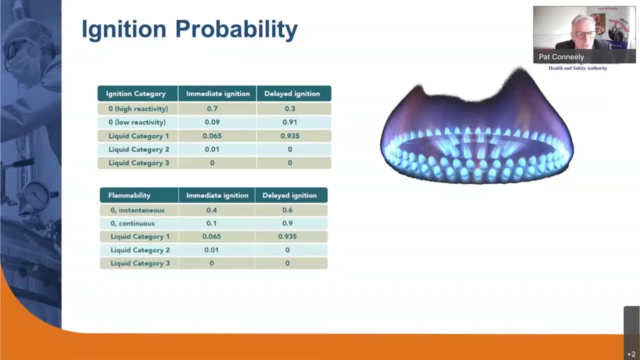 relate to transport units, as you can see there again using a similar type of methodology And also ignition probabilities for specific gases are also very similar to those of flammable liquids, as you can see there again using a similar type of methodology, And also ignition probabilities for specific 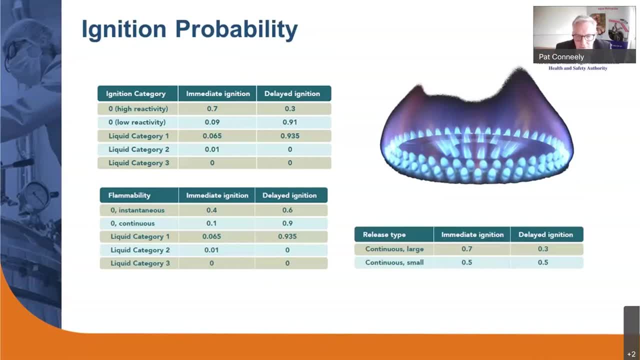 gases are also very similar to those of flammable liquids, as you can see there again, using a similar type of flammable releases at jetties, for example, And that's also the first time that's appeared in the guidance. So a very comprehensive list of ignition probabilities is provided, As you will shortly see. 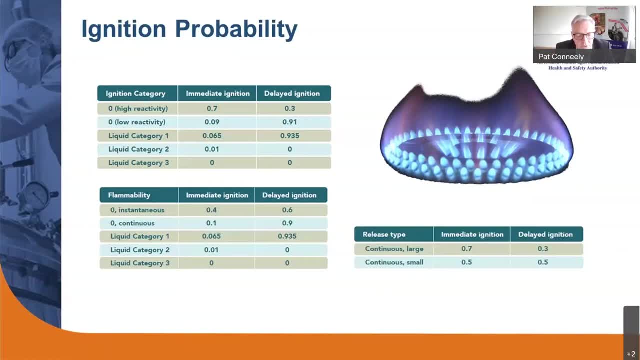 the delayed ignition probability refers to the delayed ignition branch of an event tree, But an allowance is sometimes made that some sub-branches will not result in fire and explosion. So it doesn't definitely mean that there will be an explosion event consequent on that, And that's in line with the approach in the BEVI itself. 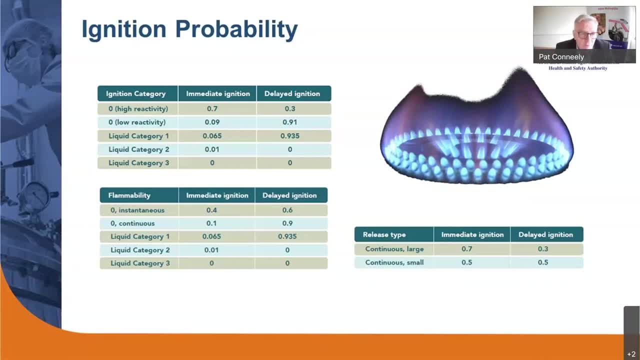 and also the methodology used in the Flemish region of Belgium, which is widely supposed to be merged and followed elsewhere. So hopefully this will all become clear when I look at event trees a bit later on. So briefly now, if I might just pause there. 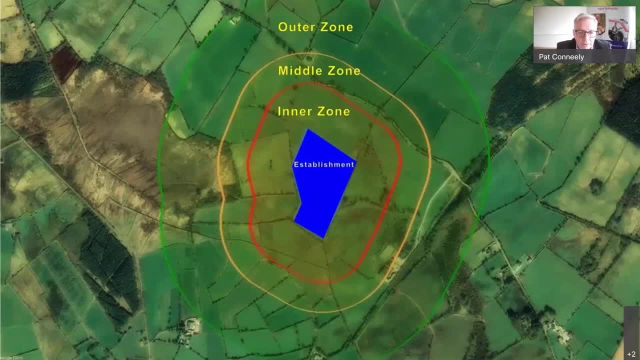 I've come to the end of my overview on part two of the guidance And we set out the approach to land use planning. It's fatality-based, And so I've tried to pin down there in part two the values of the variables that the variables will take in deriving that. 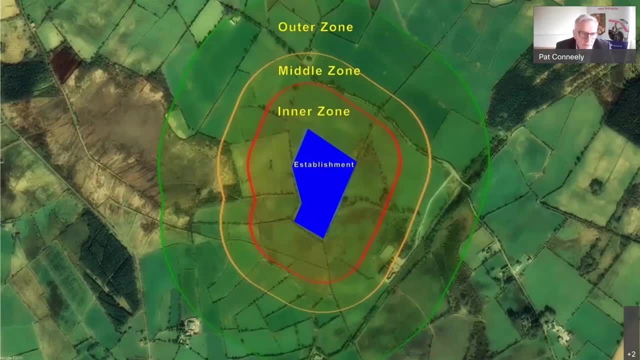 So to ensure that a consistent approach is taken erring on the conservative side, The guidance sets out the standard approach the HSA will take in deriving generic land use planning contours for planning authorities. So the final piece now is to identify the appropriate scenarios. 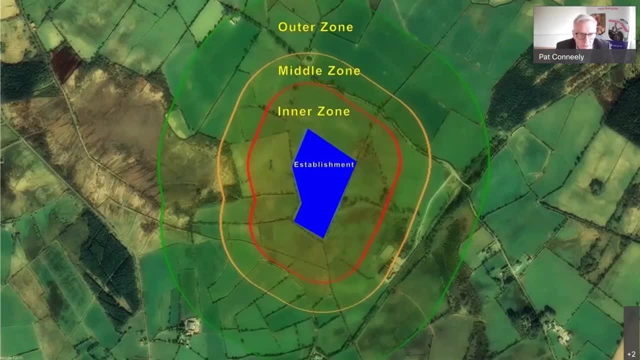 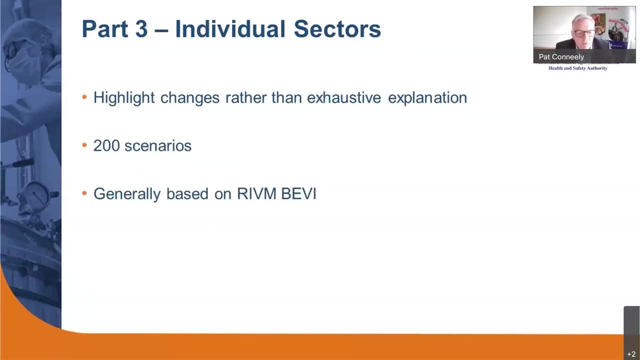 and their likelihood, And that's what part three of the guidance does. So I will try to highlight the approach taken without going into every detail. Obviously, it's extremely detailed document, and this part in particular is detailed. There's over 200 scenarios. 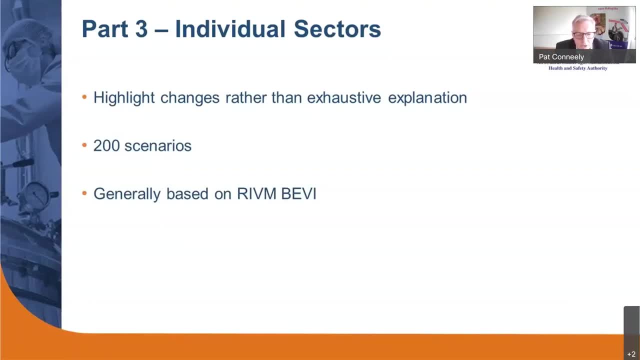 listed in part three, So I'll point out where the more important changes have been made. For this part, inspiration has been taken from the BEVI, with some tweaks here and there, And I want to emphasize this will be the standard approach to generating generic contours around. 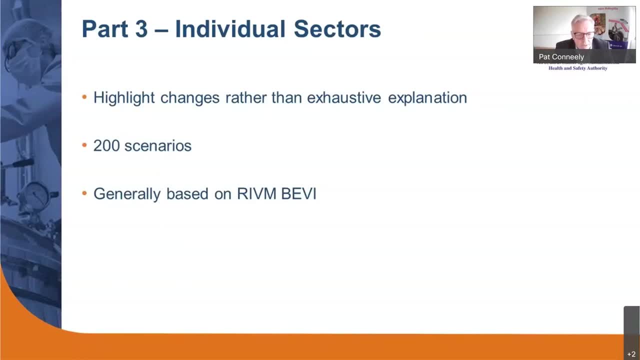 existing establishments for planning districts or cities authorities and does not preclude a more specific QRA. in the appropriate circumstances, Such QRAs should use coherent and consistent data. The authority exercises absolute discretion in deciding whether to accept such data. So the first sector that I want to have a look at is LPG. 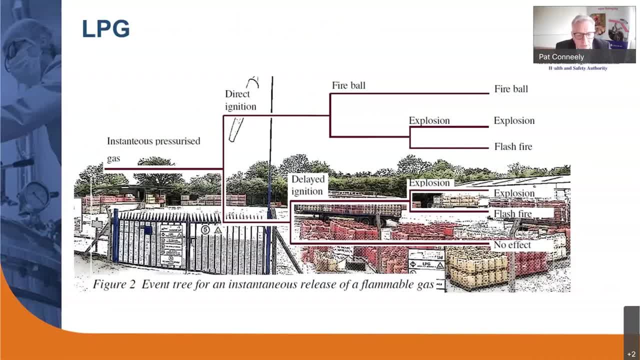 and I will use it to illustrate the general approach. This is an inventory shown there which is from the BEBI and before that it appeared in the PURPOR book, And it's for an instantaneous release of flammable gas and you can see the sub-branches for immediate and delayed 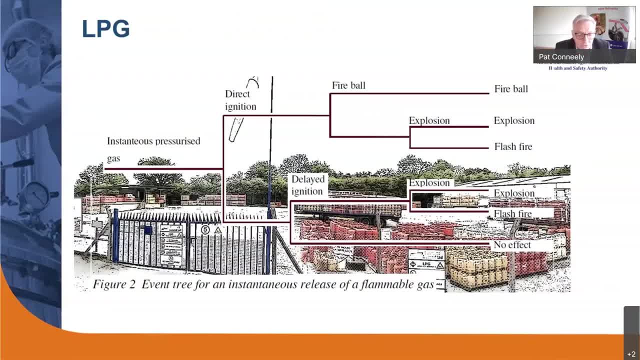 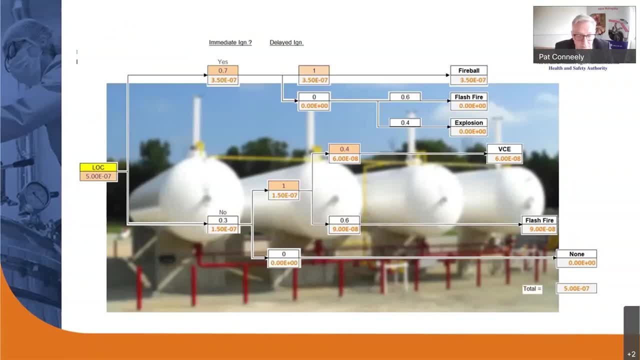 ignition and you note also that some branches result could result in no effects from delayed ignition. So the nuts and bolts. then Here is the inventory that was populated for that instantaneous release scenario. You can see the ignition probabilities for the various branches and that some end with the BEPI. 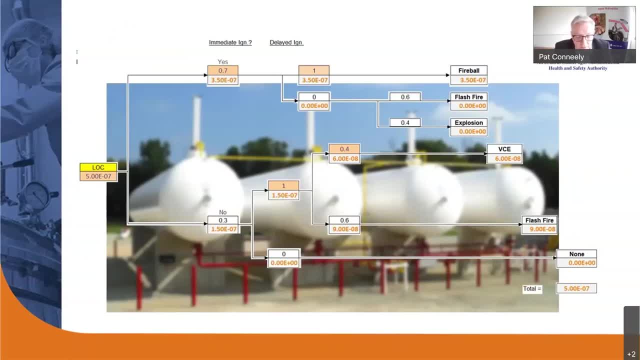 LPG is highly flammable and so is in ignition category zero high reactivity. That means an immediate initial probability of 70% and a delayed probability of 30%, And at the bottom of the slide there you can see that how data entry information has been. 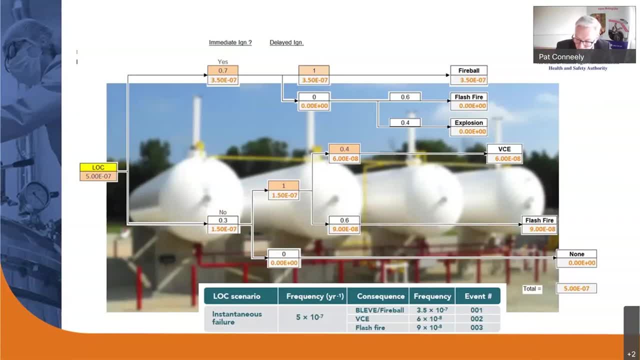 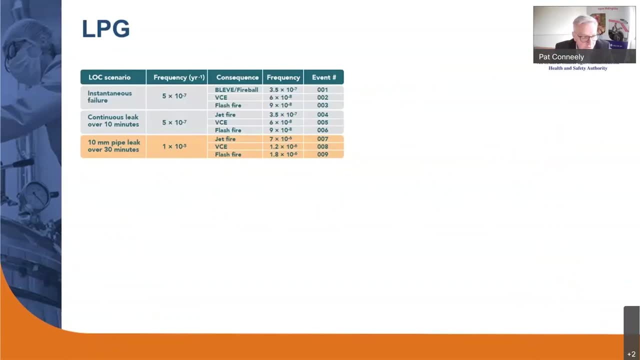 transformed into part of table 23. And you can see the full table here and that takes is taken the data from that. Now a similar approach yields the tables for the other scenarios, For the 10 mm scenario which is highlighted in orange in the first table. that means that those scenarios may only be relevant. 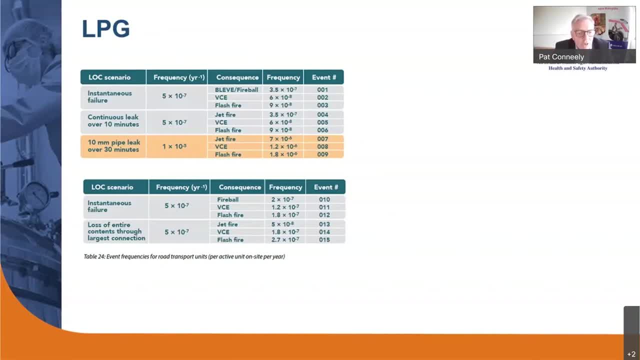 close to the establishment boundary And you will see that approach taken in some other tables. So we made these and other changes following the public consultation, where we received comments that there were too many scenarios and that the data entry was too high and that the data entry 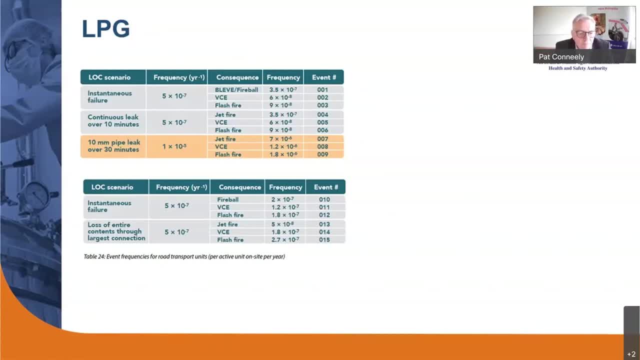 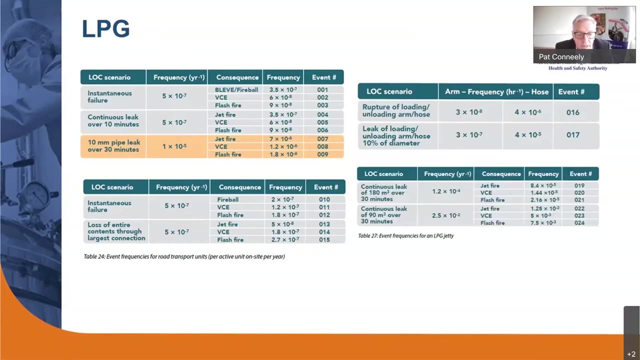 was and requesting that we just try to reduce the number. The second table there was for road transport units And we also have included now a table for loading arms and finally for jetty operations. So it's a very comprehensive coverage for the sector. now that will specify how the modeling is to be done in the standard case. 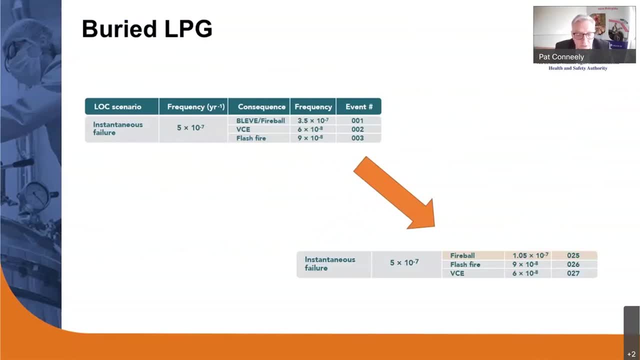 Another point to note for the sector is that explicit allowance is made for buried or mounted vessels and the reduction in blivvy likelihood. You can see that the table for buried vessels no longer includes a blivvy frequency, just a fireball frequency. The blivvy frequency now leads to no effect. That's not shown. 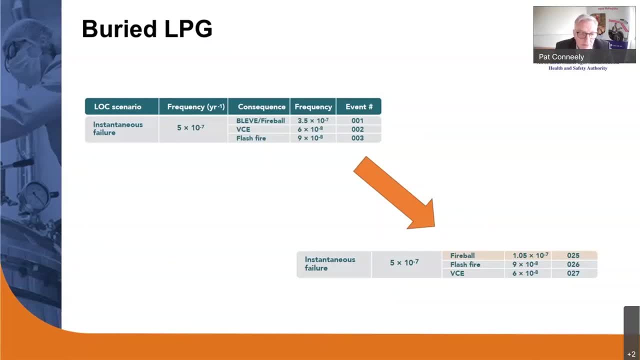 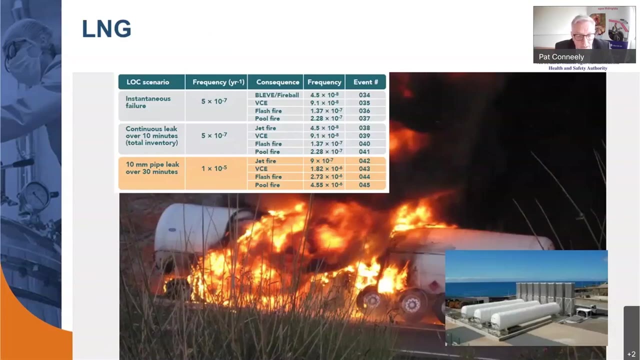 on the table because I wanted to emphasize the comparison with the standard vessels in the table above it. But it should be added in to tally up with the frequency of the scenario. Slide 23., Slide 24.. So I'll push on now to the LNG sector, which is new and developing, And again, 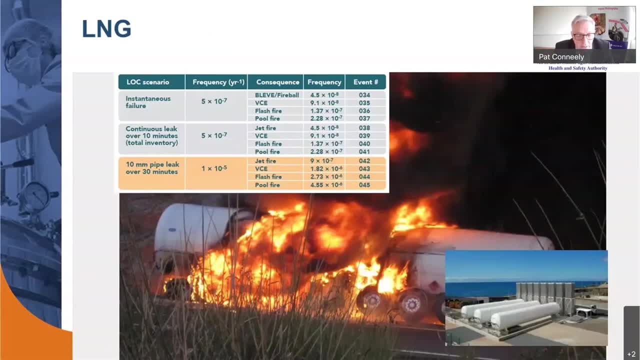 that's a new sector in our guidance And again, using event trees and the ignition probabilities in part two of the guidance, similar tables were obtained for this sector, Slide 25.. Now, because of the potential release conditions for LNG, it's stored typically at minus 160. 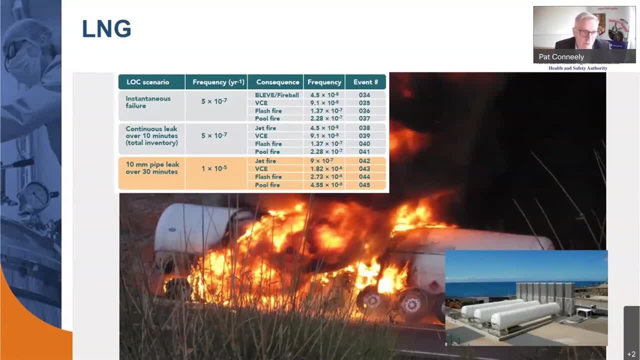 degrees Celsius and may or may not be under significant pressure, And that would in theory, depending on how it's going to be used. So pooled fire frequencies are greater than for LPG and blivvy frequencies are less. This section of the guidance is directed at smaller scale use. 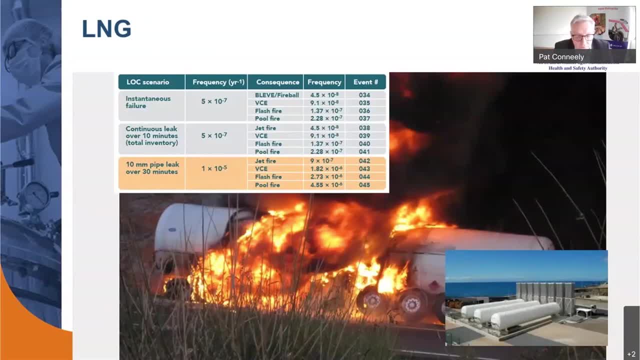 of LNG, because we have encountered a number of those arrangements at existing energy consumers and suppliers. But it doesn't cover larger facilities, particularly floating gas and floating storage for the gasification unit, Slide 26.. Floating storage units, FSUs and the like, So it's very much geared for the typical user. 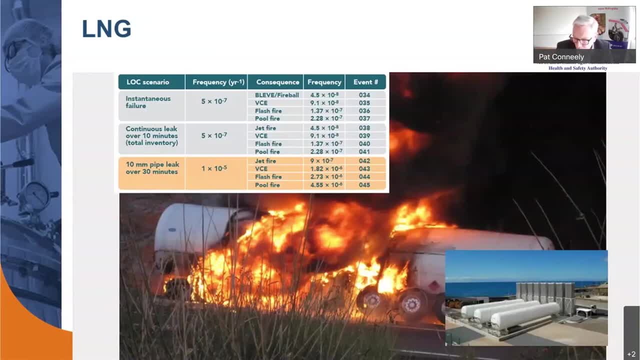 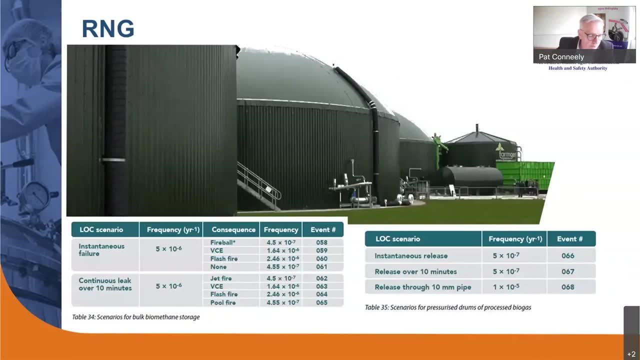 or possibly supplier arrangement that we find at the moment, Slide 27.. So we'll move on again to another sector which is for RNG. RNG stands for renewable or recovered natural gas, And this is another sector which is included for the first time in 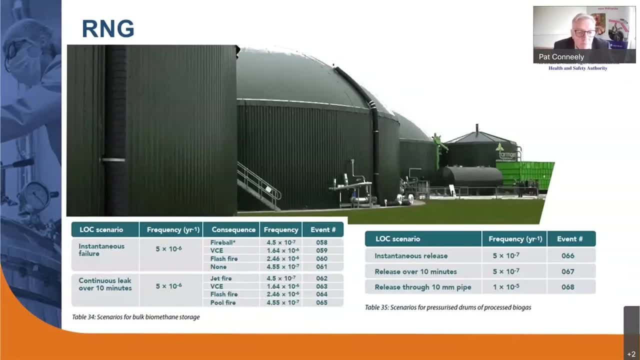 the guidance. There's not a whole lot out there to help in drawing up the tables for this. Because RNG is produced under low pressure, it was considered that fireball followed by fire would be more credible than a blivvy event, for example, And for continuous releases, jet fires were. 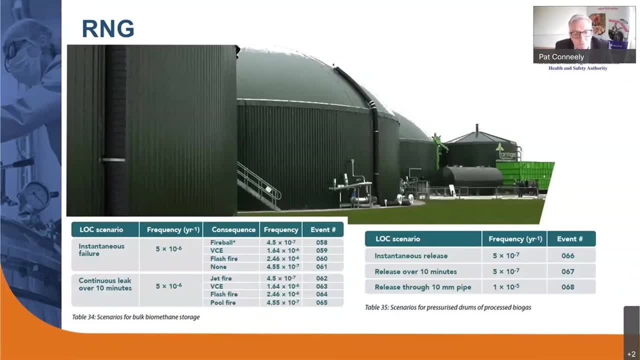 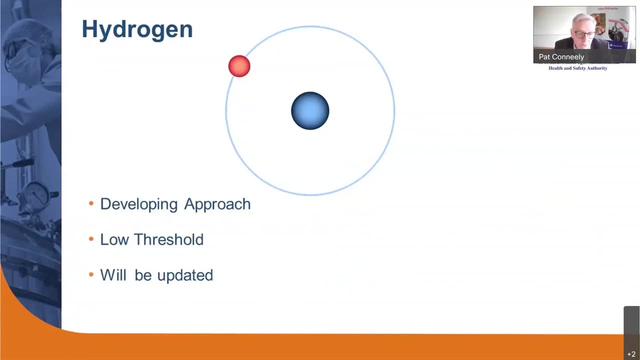 considered to have some probability, Slide 28.. Once purified, the recovered gas is pressurized into drums or cylinders, So that is also addressed for this sector, as you can see from the second table there, Slide 29.. Hydrogen sector has also been added for the first time and it's really in there as a placeholder. 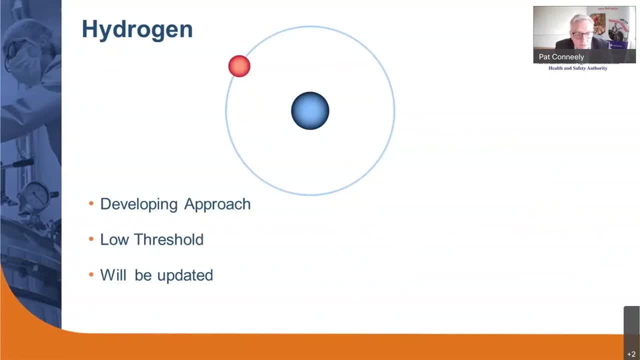 at the moment: Slide 30.. Until the end of the year, Slide 31.. Until the end of the year: Slide 32.. Until we see how the technology developed: Slide 33.. Hydrogen is a flammable pressurized gas. 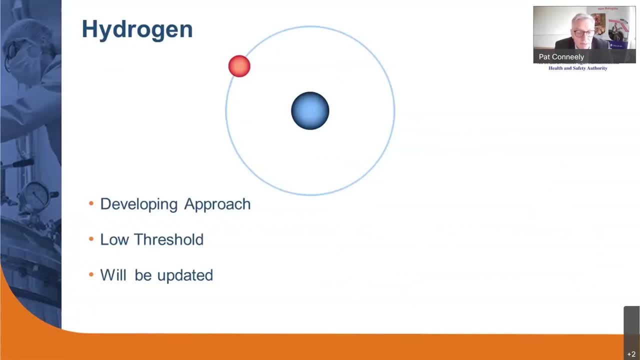 so the scenarios for flammable gases and for drums and cylinders and other sectors will be relevant and can be drawn on if more specific data is not available. But the guidance is intended that the guidance will be updated once the technologies become clear- Slide 34.. Slide 35.. 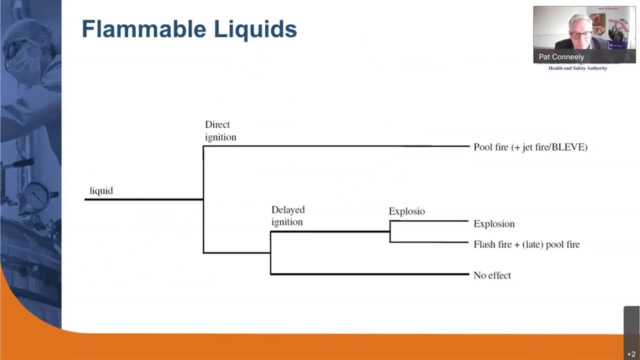 So I'll turn now to flammable liquid storage installations- Slide 36.. Slide 37. You saw in part two of the guidance that there is now a much greater discrimination between the different categories of flammable liquid, and that's also very apparent. 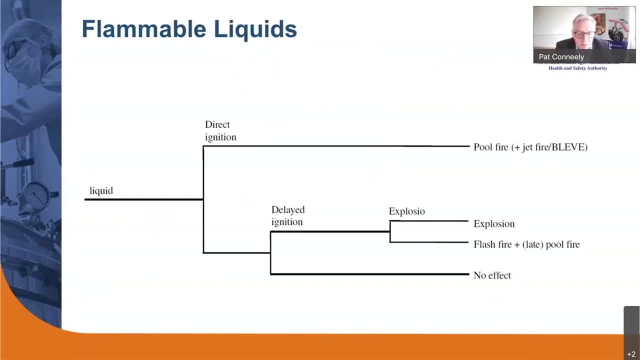 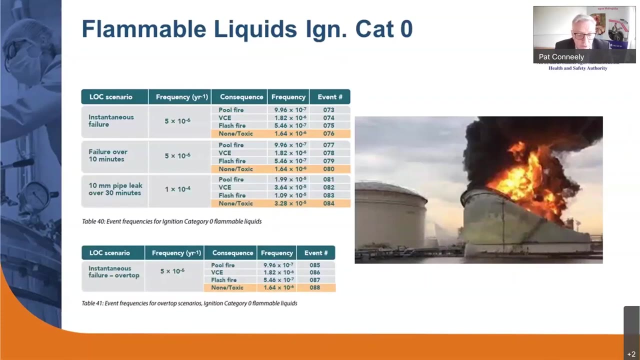 in part three. This is the base of entry from the BEVI, which is then modified to take account of the ignition probabilities of the different categories of flammable liquids. You can see here tables for liquids with low boiling points and very low flash points. 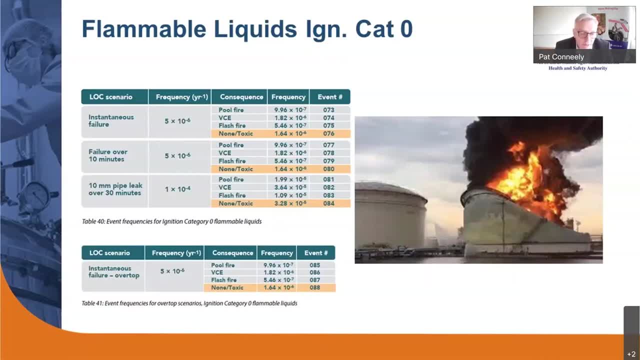 which are characterized as ignition category zero liquids. in the guidance, As you would expect, the full panoply of consequences- pool fire, vapor cloud, explosion and flash fire- are included for this category. Lines not resulting in ignition events are described as toxic or none and that 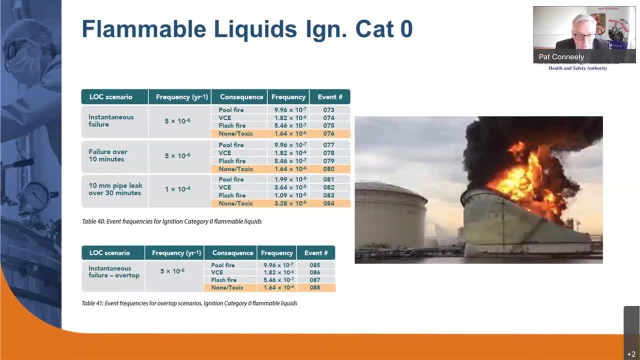 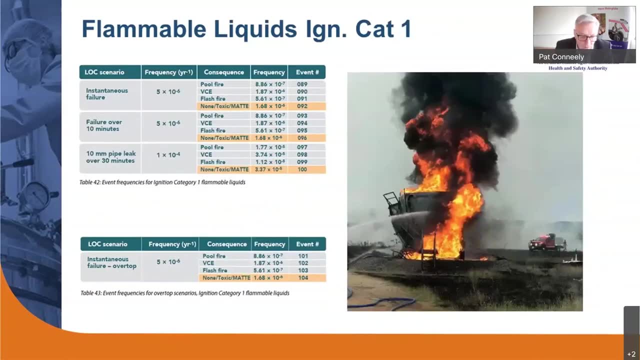 differentiates from the low reactivity flammable gases that fall into the same ignition category: Slide 38.. Slide 39. For other flammable liquids category one that fall into ignition category one, those events are are less probable and more emphasis is also given to the potential for matty events. 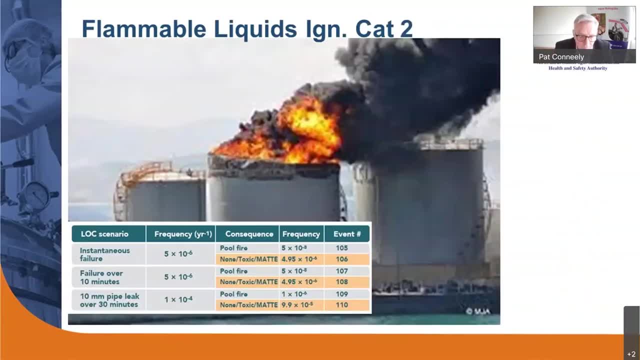 Slide 40.. Slide 41.. Second table- sorry, yep, I moved on there. So by the time we reach ignition category two, then we're just modeling pool fires: Slide 42., Slide 43. And of course they're at a reduced frequency And we also include the potential for toxic or matty. 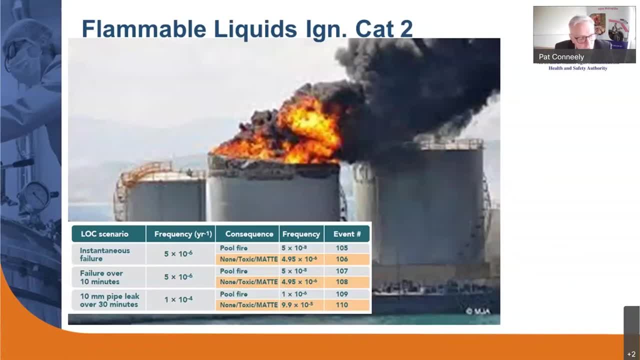 Slide 44.. Slide 45.. And then when we move on to ignition, category three, liquids, fire and explosion events are not relevant unless they are co-located with the more flammable liquids. So again, that's quite a big change from the existing guidance. 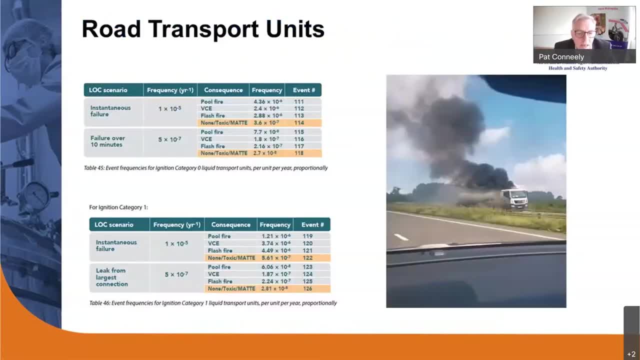 Slide 46.. Slide 47.. Another innovation for this sector is the provision of detailed loss of containment scenarios for road transport units at an establishment. Again modeled events and frequency depends on the flammable and ignition categories. Slide 48.. Slide 49. 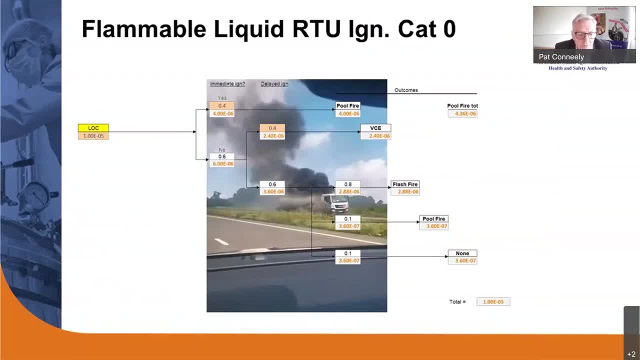 So I'll just take it through now the derivation of the tables for some road transport units: Slide 50.. Slide 51.. So we started with the basic BEVI event three and used the ignition probabilities: Slide 52.. Slide 53.. for road transport units in part two of the guidance: 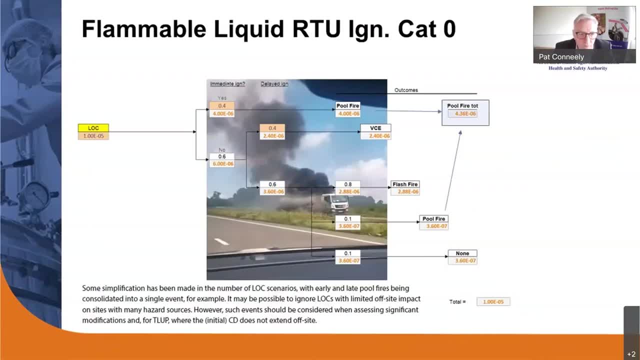 Slide 54.. Slide 55.. And we also make allowance that there's probably that some events will not result in fire explosion. Slide 56.. Slide 57.. I also want to point out something else on this tree. You recall I mentioned previously that 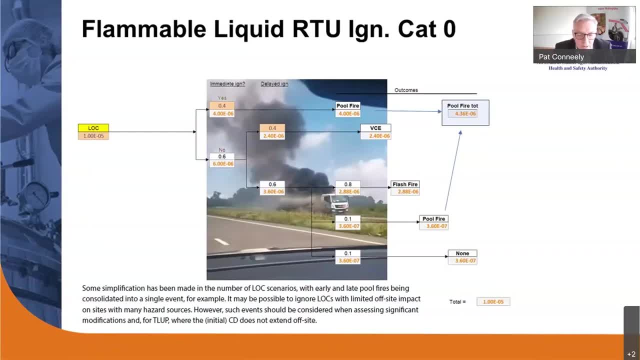 following the public consultation, we made an effort to reduce scenarios where we could. So, for example, we've done that here and maybe in lots of other trees as well, where we've combined early and late food fire scenarios into a single scenario. So, as you can see, 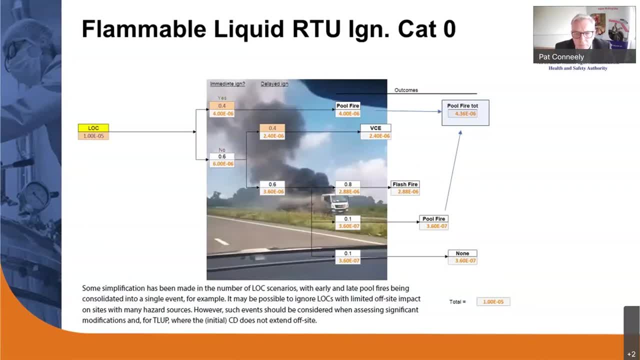 Slide 58.. Slide 59.. there showing this total cool fire probability, there is 4.36 by 10 to minus six. Slide 60.. Slide 61.. So if you actually come in and just look at the tables and try to maybe reverse engineer them, 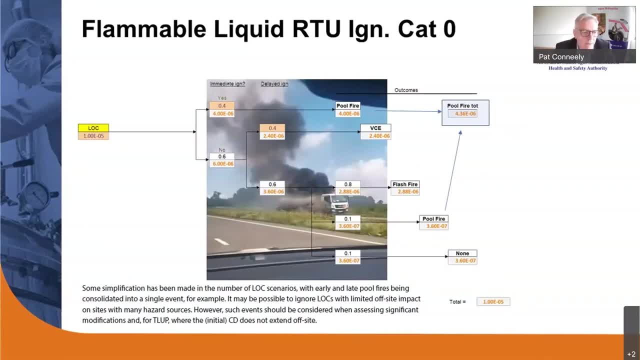 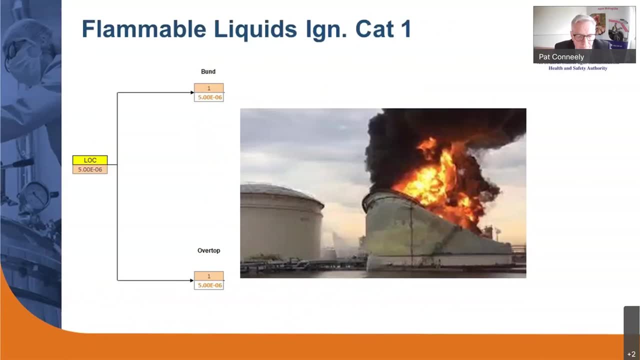 you might find that the numbers don't add up, And that's the reason why that's the case. Slide 62.. Slide 63. And again, just to illustrate the complexity involved in producing those simplified tables, let's look at the instantaneous tables. 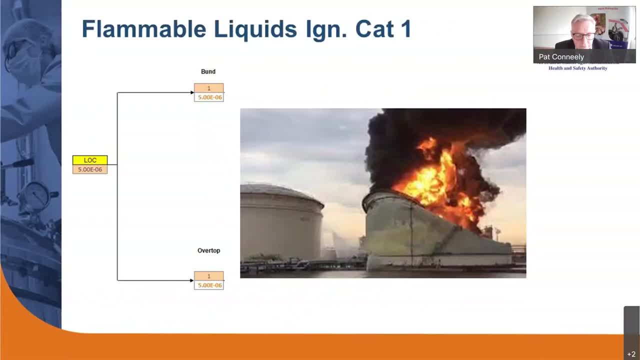 Slide 62.. Slide 63.. So this is an example of the instantaneous failure of a tank containing flammable liquid- category one- and ignition category. Slide 62.. Slide 63.. Two trees have to be considered here: One for the spill in the bund and one for the overtop event. 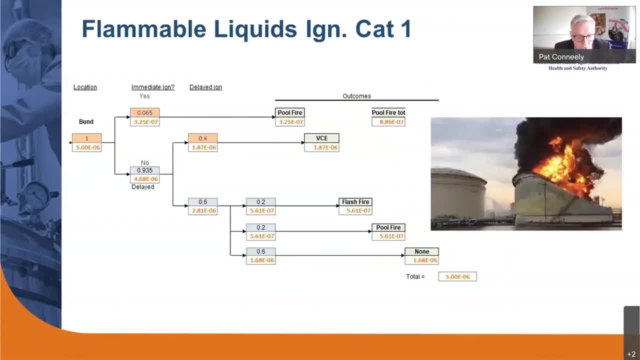 Slide 64.. Slide 65.. This is the bund event tree, The ignition category one ignition probabilities are used. Slide 66.. Slide 67.. Slide 68.. Slide 69.. Slide 69.. Slide 70.. Slide 71.. Slide 72. 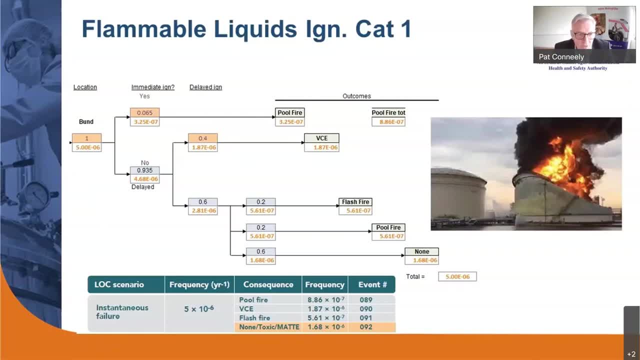 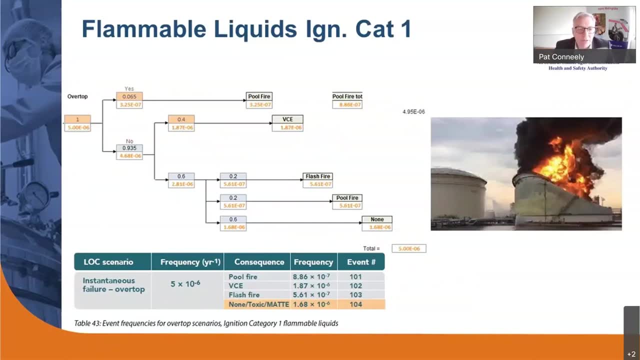 Slide 73.. Slide 73.. Slide 74.. Slide 74.. In that part of the table then describing the instantaneous failure event: Slide 75.. Slide 76.. And similarly for the overtop event tree and the resulting table: Slide 76.. Slide 77. 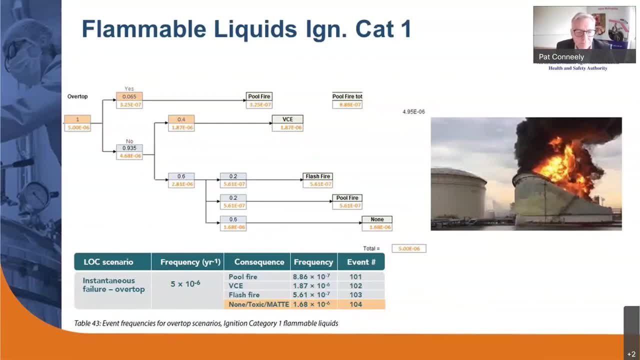 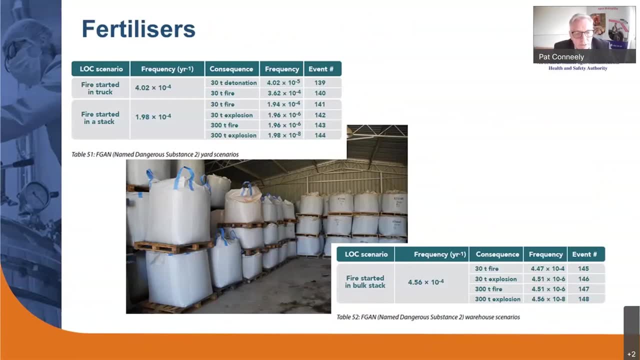 So you can see there's a lot behind those simplified tables in the guidance- Slide 78.. Slide 79.. So now I'll just move on to the next sector and that's the fertiliser sector. And there has been a significant enough consolidation of methods in for the 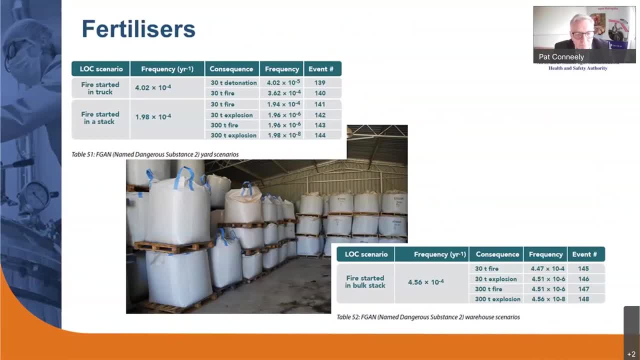 sector and a single approach is specified: Slide 78.. Slide 79.. It's explicitly stated in the guidance that applies only to ammonium nitrate name substance two fertilisers, which is the type of fertiliser we usually encounter in Ireland. Slide 78.. Slide 79. 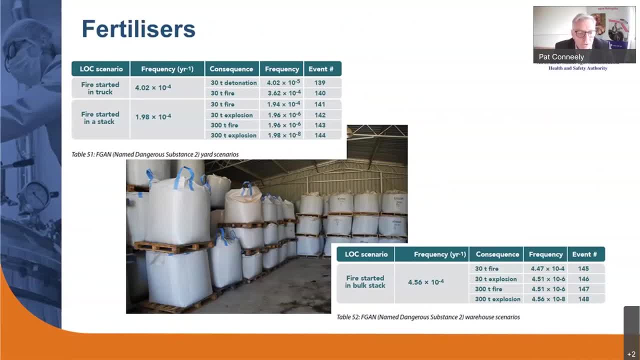 Model scenarios will be for fire and explosion on trucks and in the yard, stacks stored in the yard and for bulk storage in warehouses. Slide 78.. Slide 79.. 300 tonne detonation events are included, but they're at a very low frequency. 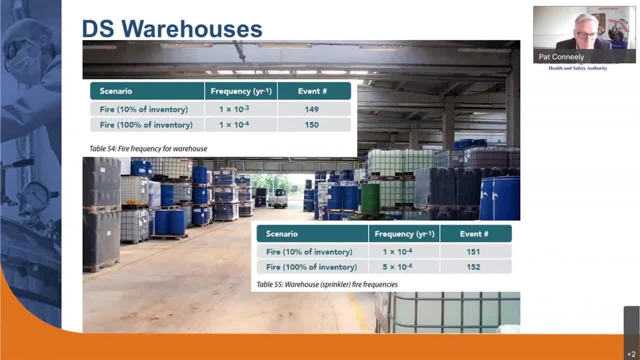 Slide 78.. Slide 79.. For dangerous substances warehouse, there haven't been too many changes for that sector. Slide 78.. Slide 79.. One point to note is that now there is a clear allowance for frequency reduction for small and large warehouse fires where sprinklers are installed and operational. 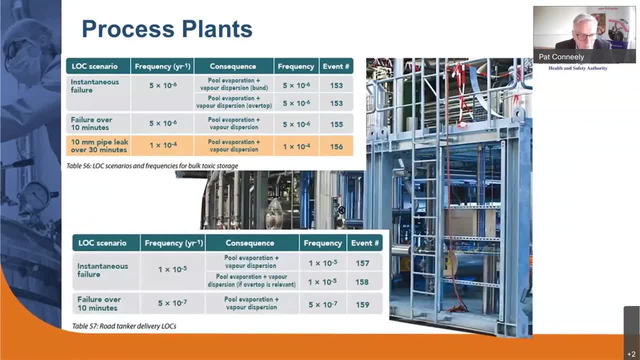 Slide 78.. Slide 79.. For process plants, a table of loss of containment events involving bulk storage of toxic liquids, which was absent in the previous revision, has now been added. Slide 78.. Slide 79.. Also, events involving road transport units have now been specifically included. 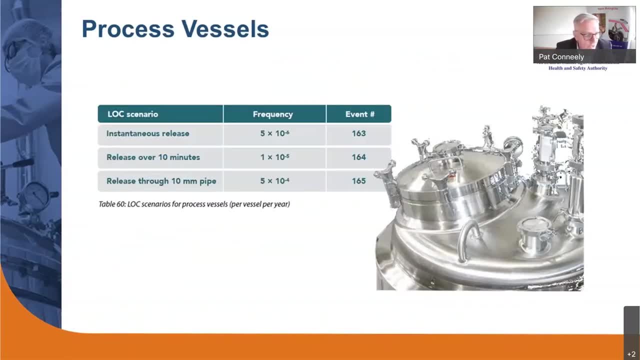 Slide 78.. Slide 79.. And the approach to process vessels has been set out. Slide 78.. Slide 79.. The guidance recognises that releases may occur at elevated temperature or pressure. Slide 78.. Slide 79.. A simplified approach ignores explicit consideration of the many sources of 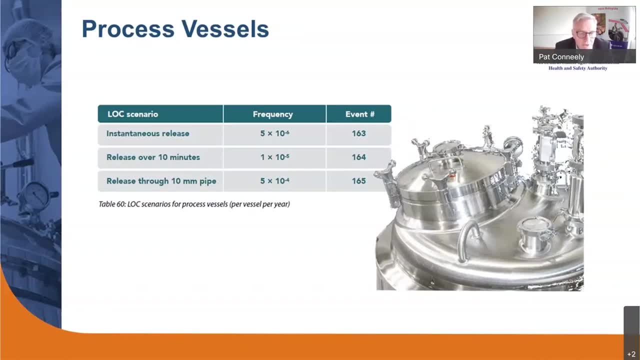 potential release pipes, pumps, compressors, heat exchangers and so on- and instead increases the frequency of releases from the process. vessel Slide 78.. Slide 79.. The loss of containment figure for a vessel can be multiplied by the number of active. 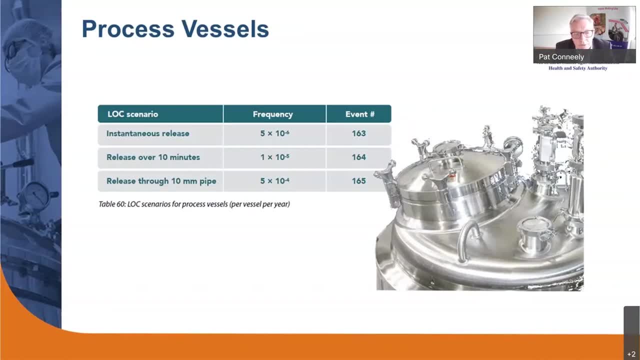 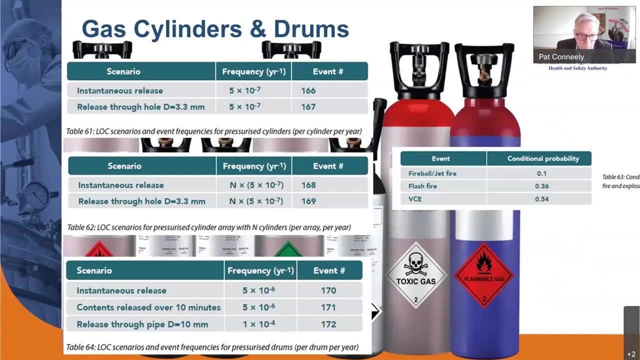 vessels in the reactor hall or building: Slide 78.. Slide 79.. And an increase in frequency is also made for vessels carrying out exothermic reactions- Slide 78.. Slide 79.. The storage and use of gas cylinders and drums has also been revamped. 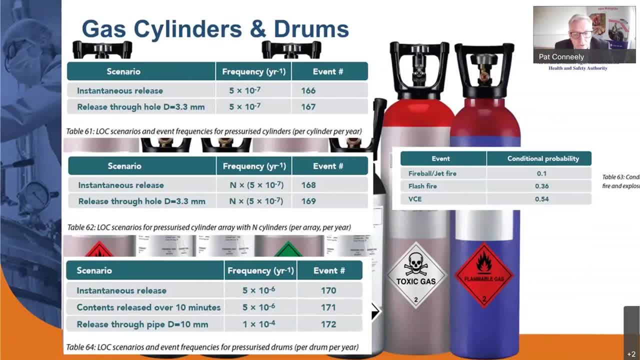 Slide 78.. Slide 79.. Differentiation is now made between cylinders, which are containers with a volume of less than 150 litres, and drums- Slide 78.. Slide 79.. Arrays of cylinders are now explicitly addressed- Slide 78.. Slide 79.. 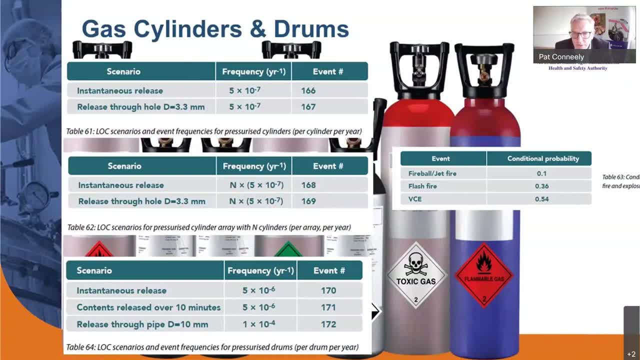 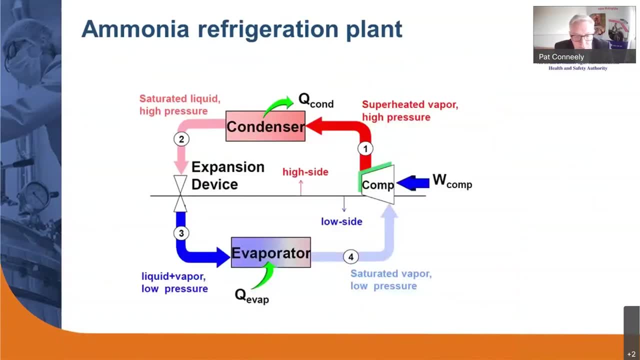 And conditional probabilities are set as shown there in Table 63,, which is included on the right- Slide 78.. Slide 79.. A morning air refrigeration plant has been included for the first time- Slide 78.. Slide 79.. 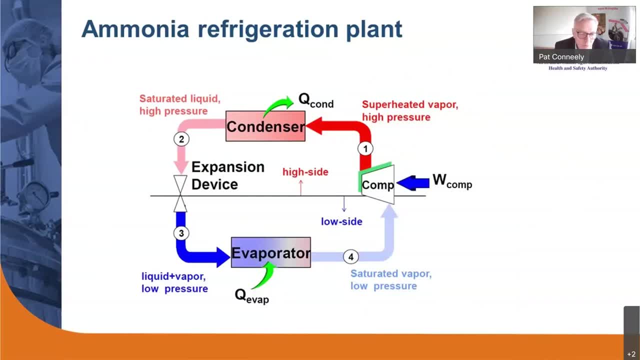 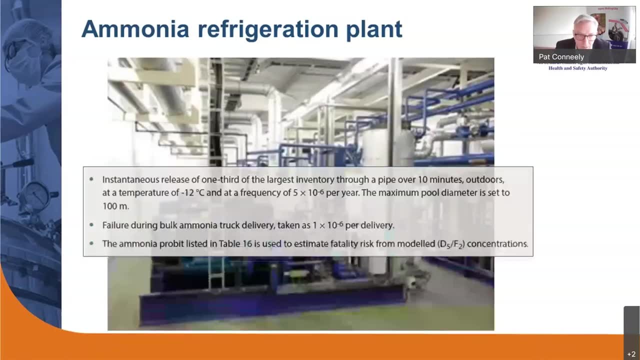 And given the different phases in the refrigeration process, with high and low pressures and high and low temperatures, finding a simplified approach for the standard LEP model was not easy- Slide 78.. Slide 79.. But we did identify a reasonable approach, which is spelt out on this slide. 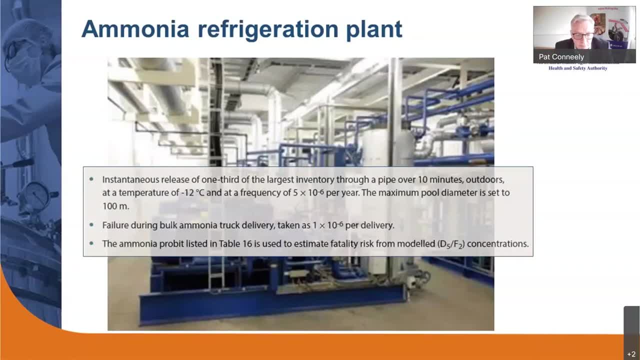 Slide 78.. Slide 79.. And it involves an ammonia spill in pipework external to the building, so outdoors, at a temperature of minus 12 degrees Celsius and with the maximum pool size possible of 100 metres diameter. Slide 78.. Slide 79.. 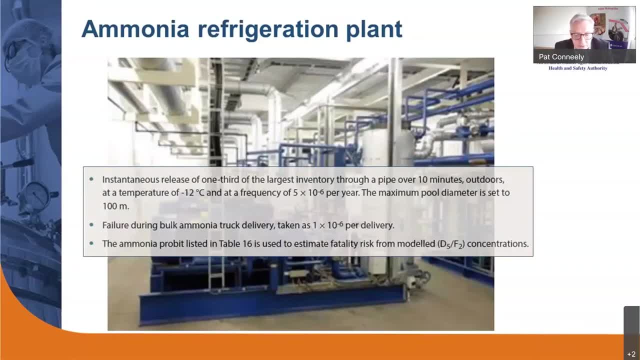 And the probit then would be taken from the toxic probit table that I referenced earlier- Table 16, and that would be used then to establish the fatality levels in D5 and F2 conditions- Slide 78.. Slide 79.. 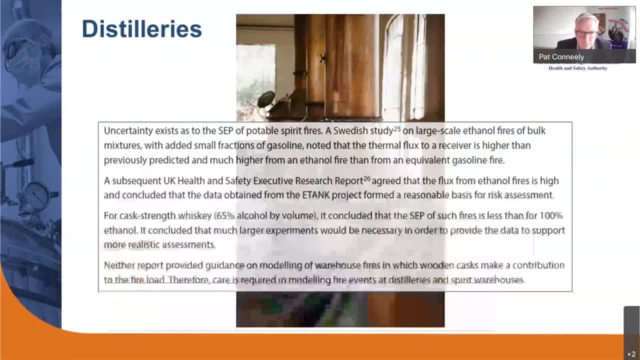 Distilleries and spurt maturation warehouses are explicitly included for the first time as well in the guidance, Slide 78.. Slide 79.: The approach to modelling of ethanol fires is not firmly established. Recent publications which you can see there: I've referenced Swedish study and an ETag. 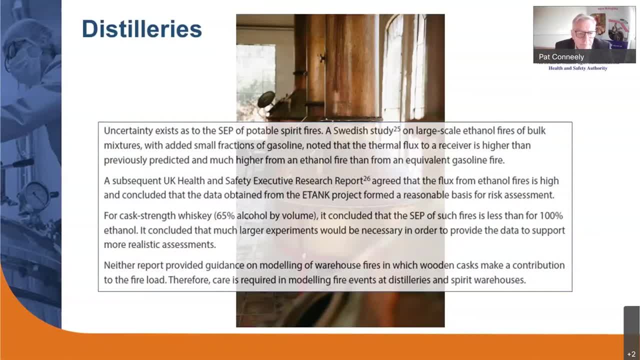 safety executive research project as well, have indicated that the surface emissive power for ethanol fires is low: Slide 78.. Slide 79.. It's greater than for gasoline and as it burns with a clear flame, the level of such obscuration is probably minimal: Slide 78.. Slide 79.. 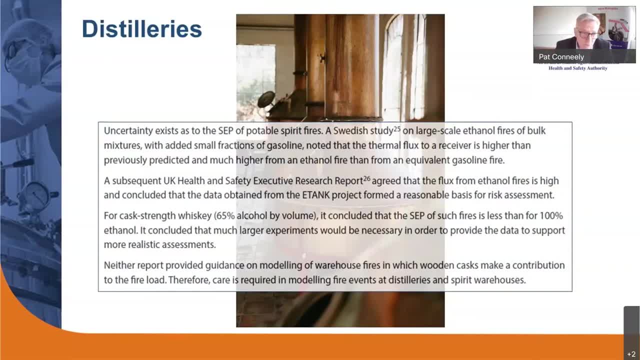 So a high surface emissive power is assumed in the standard model, Slide 78., Slide 79. Now, on the other hand, allowance is made for aqueous solutions and cast strength whisky, which are obviously much lower strength than 100% ethanol and therefore that has to be factored in. 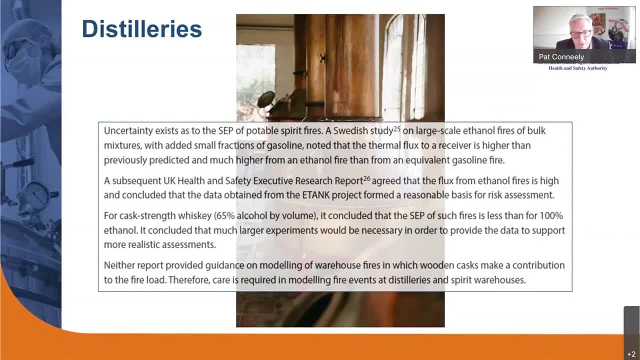 Slide 78.. Slide 79.. On the other hand, warehouse fires are modelled conservatively due to the uncertainty. Slide 78., Slide 79.. So, for example, in the case of aqueous solutions and cast strength whisky, the standard model would require a certain contribution of wooden casks. 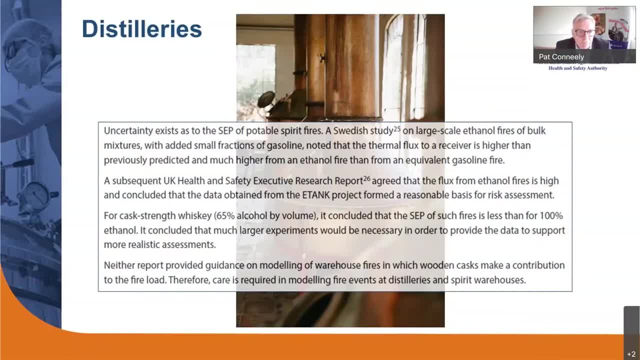 Slide 78.. Slide 79.. And you know again, we emphasise, this is for the standard model for QRAs: Slide 78.. Slide 79.. Obviously, a different approach could be taken, but we would require extensive justification for the use of lesser figures. 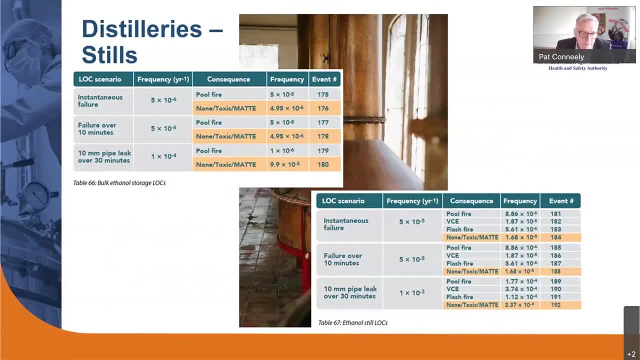 Slide 78.. Slide 79.. Ethanol is flamboyant liquid category two with ambient temperatures and the bulk ethanol scenarios reflect that Slide 78.. So that's in table 66.. Slide 78.. Slide 79.. Slide 78.. Slide 79. 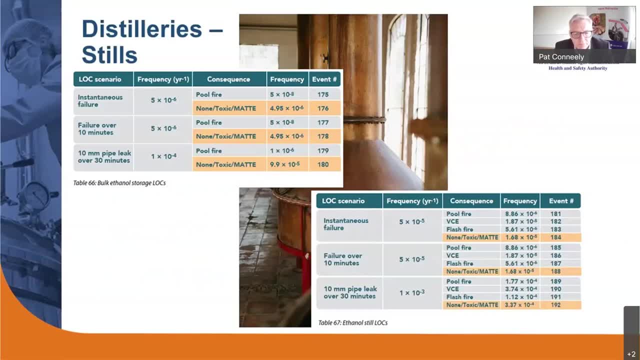 However, ethanol is at elevated temperature in a still and those scenarios are similar to a flamboyant category one: Slide 78.. Slide 79.. So again, a simplification is applied and loss of containment events for re-boilers pumps. 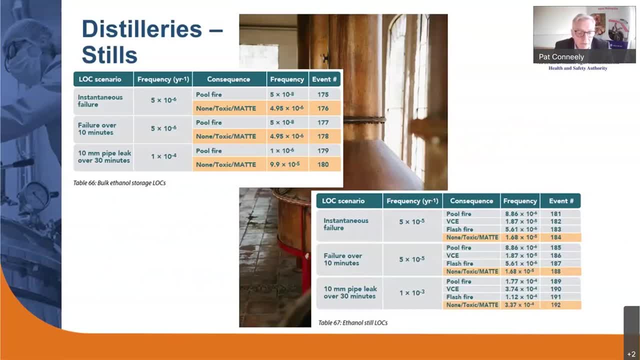 condensers and so on are reflected in the failure frequencies for the still loss of containment events, as can be seen in table 67.. Slide 78.. Slide 79.. For warehouses, lower start fire start frequencies are used and that reflects the high level. 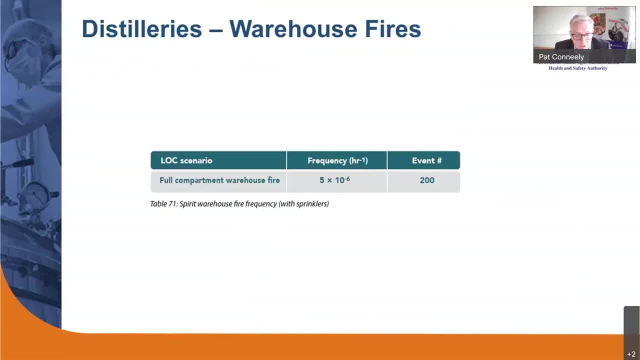 of security at these sites: Slide 78.. Slide 79.. And credit is also given for the use of sprinklers. but I should point out there's an error in that table, which should be: figures should refer to per year and not per hour. 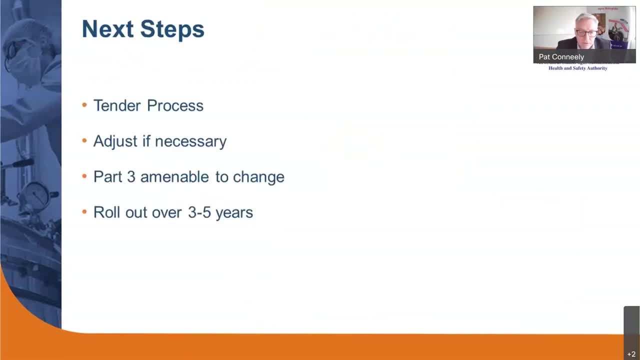 Slide 78.. Slide 79.. So I might step back now from all the technical detail and just to look at the bigger picture. Slide 78.. Slide 79.: The standard approach to be taken for the generation of technical land use planning contours. 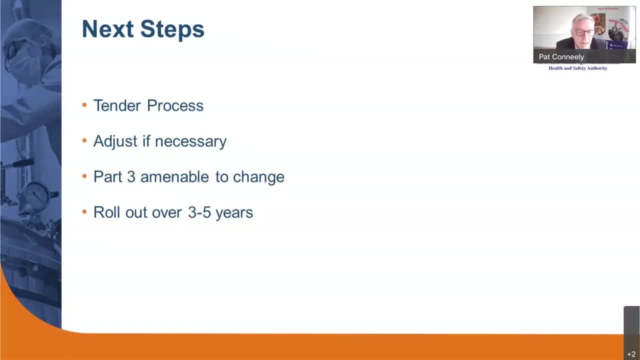 for planning authorities- Slide 78.. The standard approach to be taken for the generation of technical land use planning contours has been set out in the guidance and it does make a number of simplifications- Slide 78.. Slide 79.. And that ensures that a robust approach will be taken and the analysis will be carried. 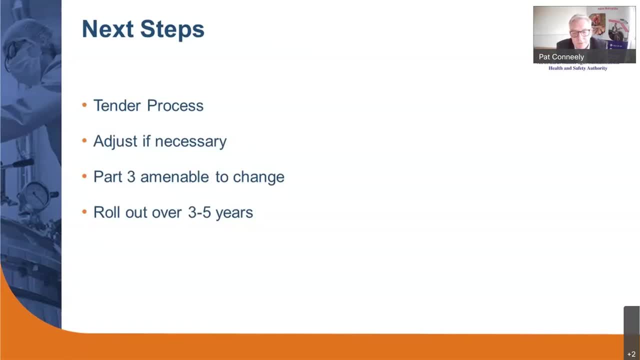 out efficiently and at a reasonable cost. Slide 78.. And, as Eisa mentioned already in her presentation, the costs will be borne by the operator, as set out by the Coma Regulations of 2015.. Slide 78.. Slide 79.. 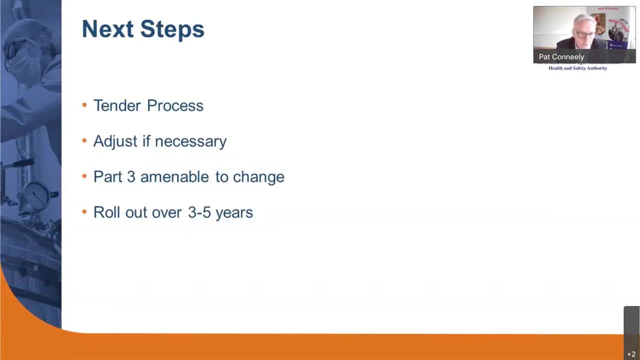 And we are tendering externally for this and the tendering process has commenced- Slide 78.. Slide 79.. And when a successful tender is appointed, I think any kinks in the approach would be ironed out at that stage, if there are. 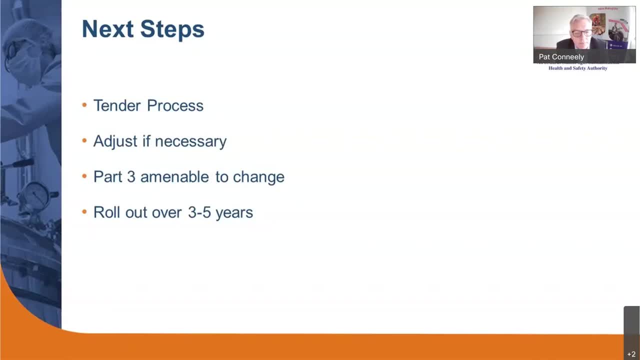 any in there. Slide 78.. Slide 78.. Slide 79.. Part 3 of the guidance is amenable to technical change and it's explicitly stated in there, in the earlier parts of the guidance, that Part 3 can be changed without further recourse to the board. 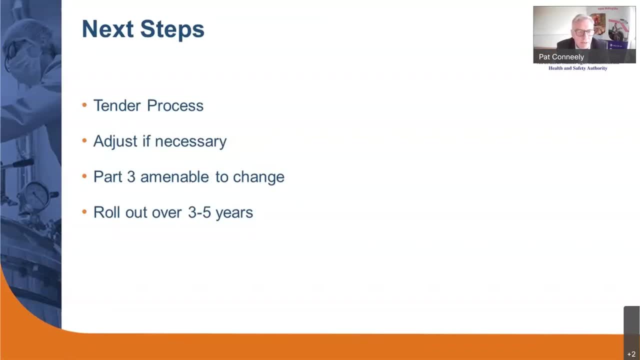 Slide 78.. Slide 79.. So it does allow us to make practical changes as we proceed and if there are any inconsistencies. as well as that, if new technologies develop- and we pointed out earlier in some of the sectors we're still looking at the technologies that might come in and how that might be applied. 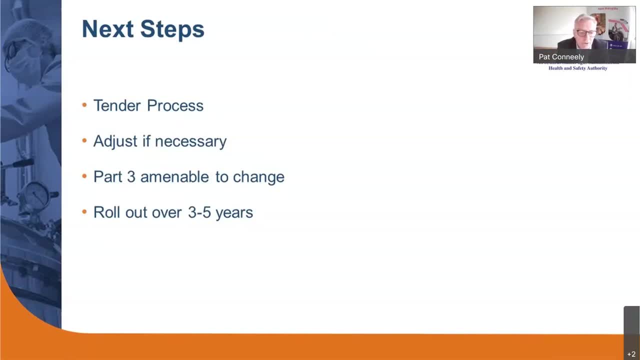 in Ireland So they can all be incorporated in the future in a much simpler process but shorter process too, hopefully, Slide 78.. So in terms of the actual rollout of the generic advice to the planning authorities, as Eisa said, it's difficult to say how long it's going to take, but certainly it would be. 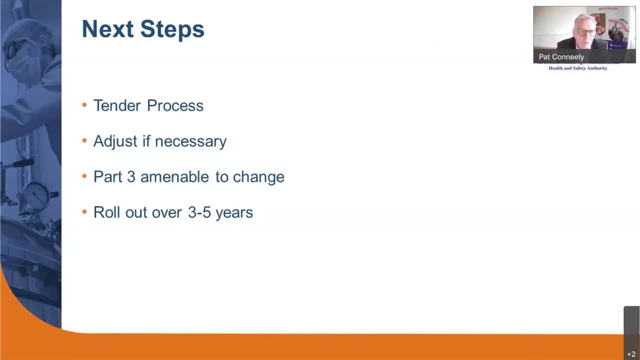 nice to get it done in three years and that would probably be the optimistic end of the spectrum. Slide 78.. Slide 79. But it could be up to five years. but I suppose, given that land use planning provisions have been in place for more than 20 years now and we still have had a lot of difficulty in rolling out, 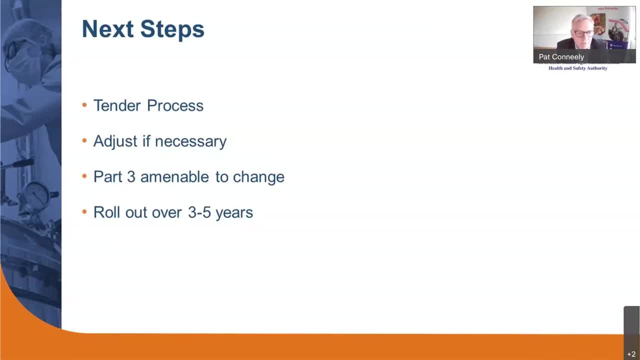 it's worthwhile, I think, now to try and get this done, and if it does take even a few years, at least at the end of that it'll be done for all sites. Slide 80.. Slide 81.. So I'd like to wrap up this section with a few final words. I've emphasised several points in 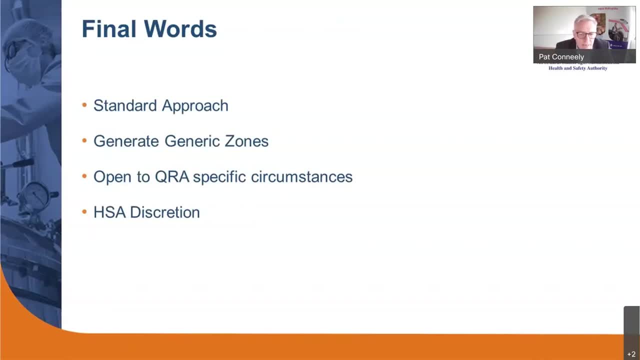 my presentation that the guidance describes a standard approach. That is the approach the authority will take in developing generic technical land use planning contours. that will be provided to planning authorities- Slide 82.. Quantified risk assessments can be submitted by operators in relation to significant modifications. 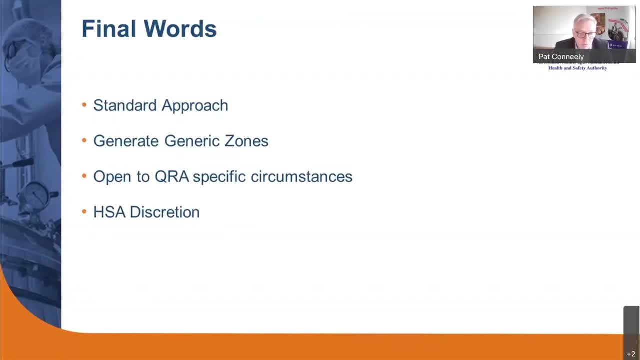 or for new establishments or by developers in support of development in the vicinity of such establishments and such careers will be examined by the authority and may be accepted as representing a more accurate assessment. Slide 83.. Slide 81. Accurate estimation of risk, but this will be at the discretion of the authority.